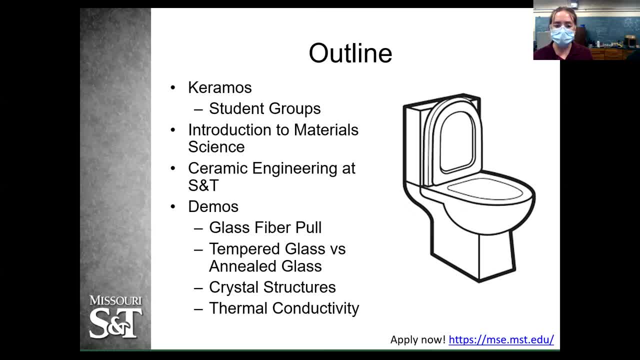 I'll give you a little bit of an overview into the student groups we have here on campus in the Ceramic Engineering Department. I'll give you a brief introduction to material science as a whole, and then I'll go into a deeper analysis into what ceramic engineering is. 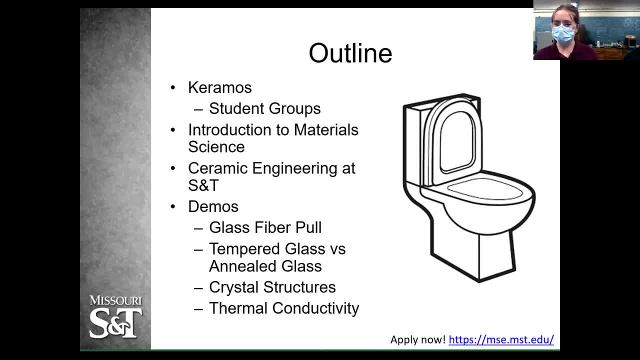 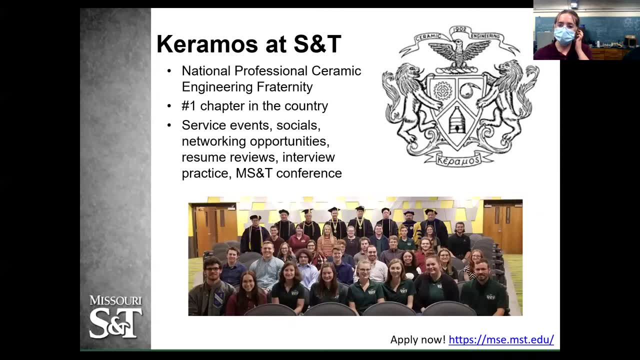 And then I'll get right into some demonstrations to show you guys some of the really cool applications for ceramics. So, like I said, we're a part of CARAMOS, We're the National Professional Ceramic Engineering Fraternity and this chapter at Rolla is the number one chapter in the country. 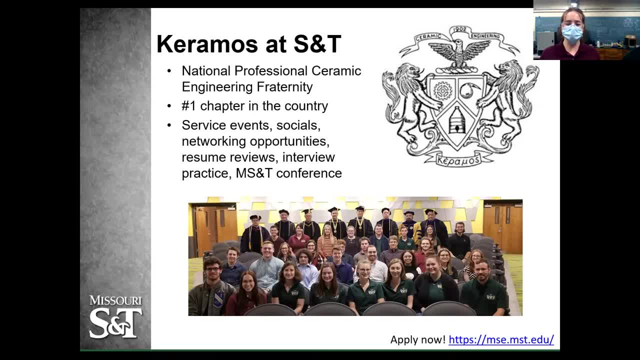 And the way they decide. that is based on things like outreach, things like this, how we support our department, how involved we are with each other, stuff like that. So across the entire country, our chapter is number one, And what comes along with being in CARAMOS is there's a lot of service events you can get involved in. 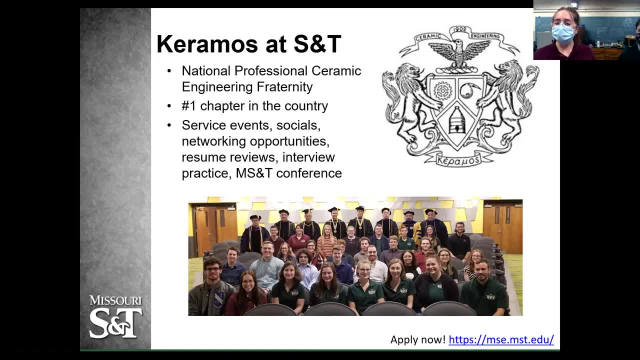 There's socials So you can get to know the people in the department better. There's lots of networking opportunities. A lot of alum come back and if they're part of CARAMOS, that's something you can start a conversation with them about. 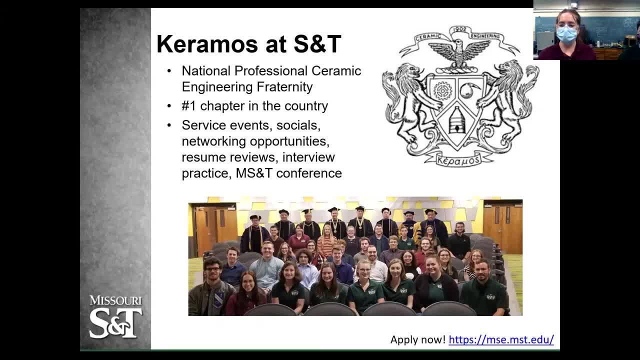 We do resume reviews all the time, So if you've got a resume that you need checked over, send it to anyone in CARAMOS- they'll look it over. We also do lots of interview practice, especially around career fair time, So that's really helpful. 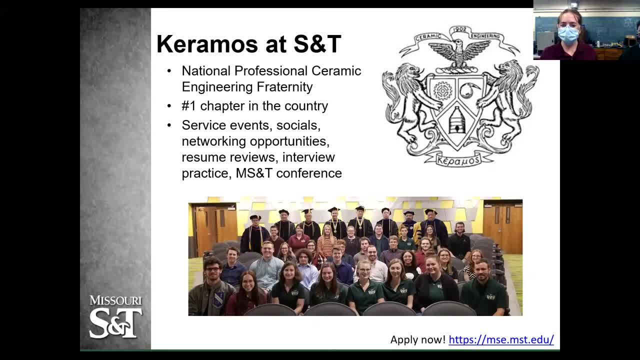 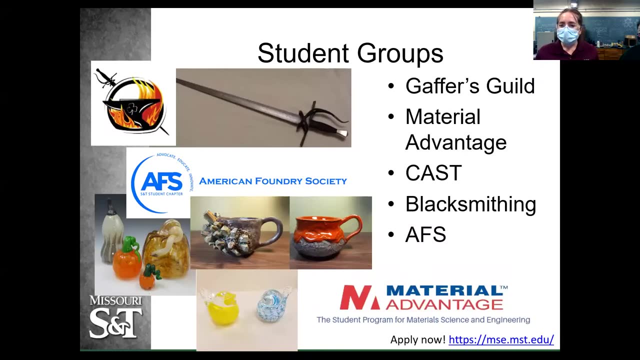 And we also have the MS&T conference every fall, which is just a big conference where ceramic engineering and metallurgical engineering departments around the country come together and do fun competitions to show off the cool things that materials can do. So the student groups we have in our department include Gaffer's Guild, Material Advantage, Cast and Blacksmithing and AFS. 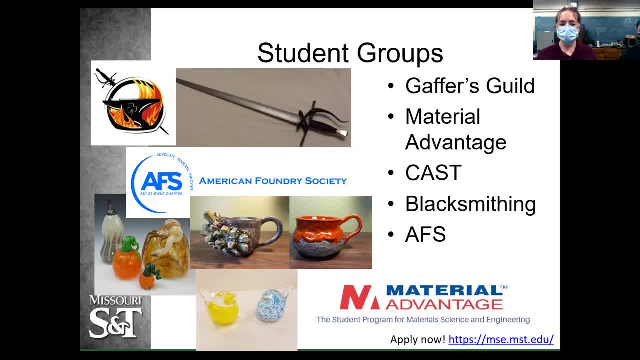 So Gaffer's Guild is our glassblowing club. We do have a. We have a full hot shop on campus. So these pictures down here, these were made on campus by students, So it's really cool. There's a class you can take to learn the basics. 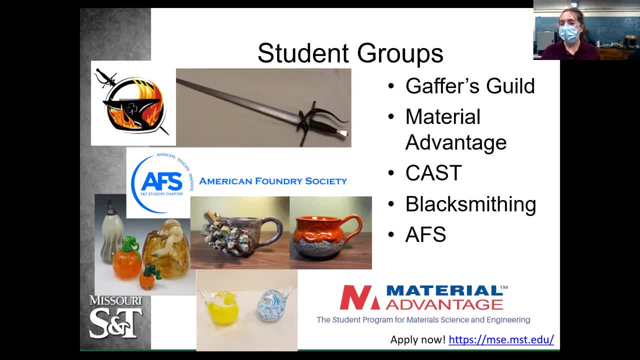 At the end of the class you can make a bunch of like paperweights and cups And then after that you are in Gaffer's Guild and you can go in anytime and start making stuff, blowing glass. We also have Material Advantage and that's kind of the overarching department organization. 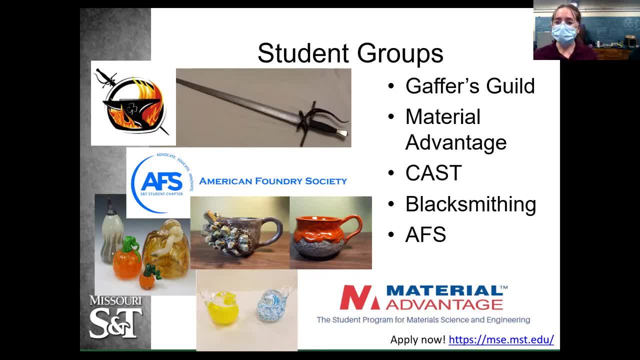 So that includes both ceramics and metallurgy. We also have We have Cast, which is ceramic artists of S&T, So they do stuff like this. They do lots of ceramic pottery and stuff like that. So that's a newer one. That one's really cool. 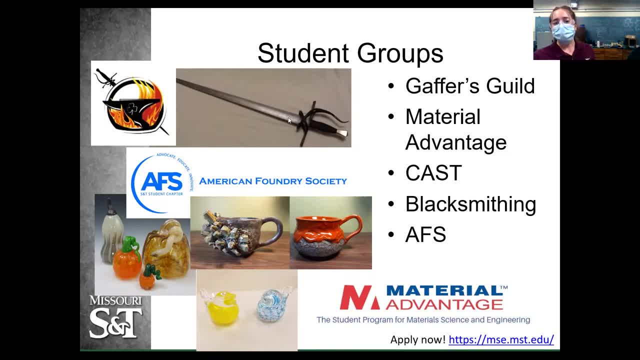 Really excited about it. We also have a blacksmithing club, So anything you can do to blacksmith- I don't have any experience with that because I'm ceramic, So but we do have blacksmithing. And then AFS is the care most version for the metallurgical engineers. 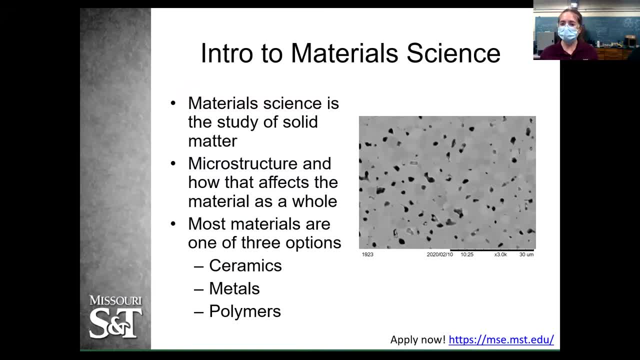 So brief intro into what What material science is. it's the study of solid matter And what we do as material scientists is we control the microstructure of materials and try to manipulate that so we can affect the properties of the material as a whole. 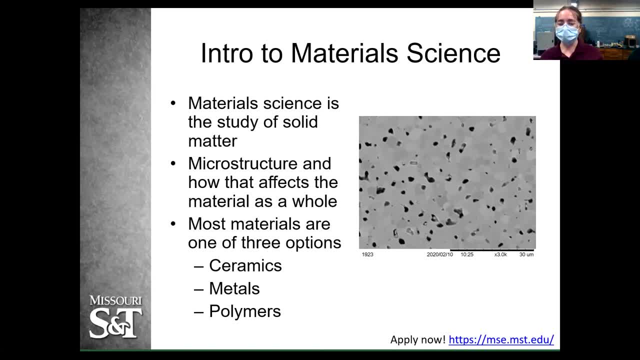 And most materials are one of three options: ceramics, metals and polymers. And, like I said, we have ceramic engineering and metal or metallurgical engineering here at S&T, And then we also have a material science engineering graduate degree And that's, that encompasses both of those. 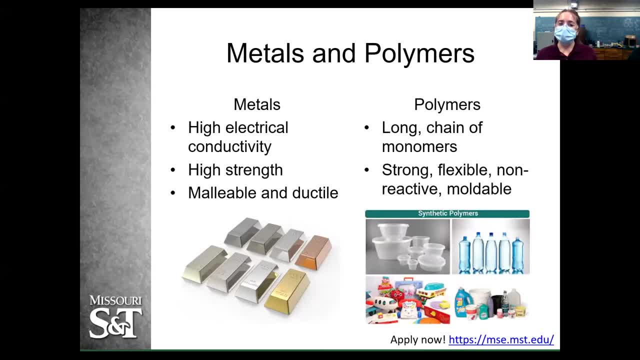 So that's the study of solid matter. So brief overview into what metals and polymers are. the staples of metals I'm sure you all know they're very electrically conductive, they're very high strength, they're malleable and ductile. 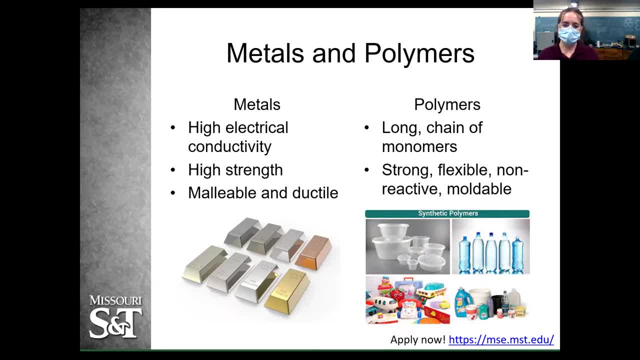 And if I asked you to come up with an example of a metal, I'm sure about all of you will be able to come up with something right off the top of your head. Polymers consist of long chains of polymers and those are your things, like plastics, foams, styrofoams, those kinds of things. 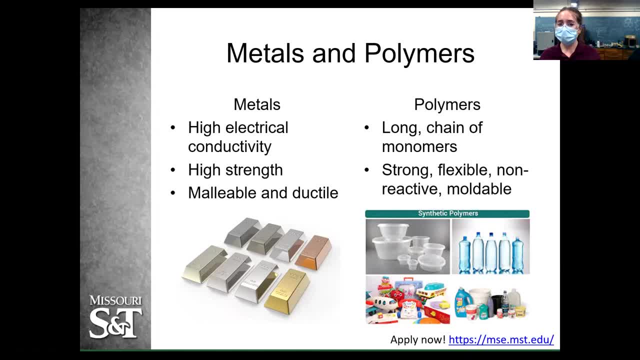 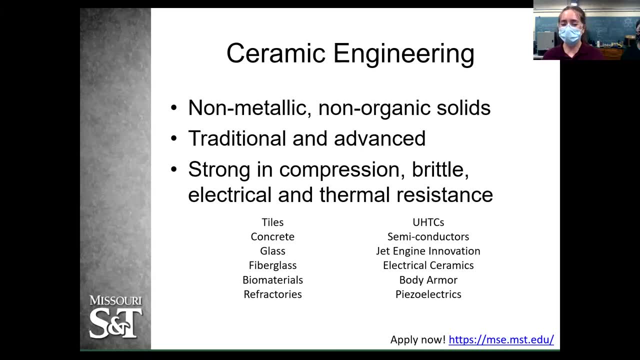 So we don't really deal with that here, But that is another branch of material science. And so here's the good stuff: ceramics: We deal with non-metallic, non-organic solids. There's two types of ceramics, including traditional and advanced. 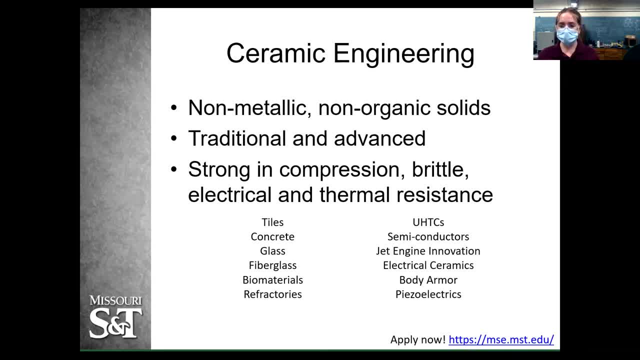 And the staples of ceramics is that they're really strong in compression, really really weak in tension forces. They're very brittle but they're very electrically and thermally resistant. So down here I've just got a bunch of examples. 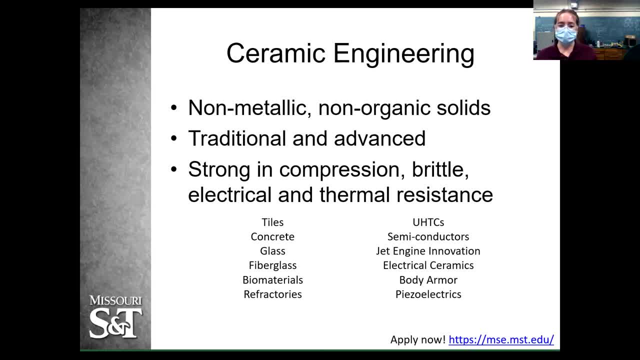 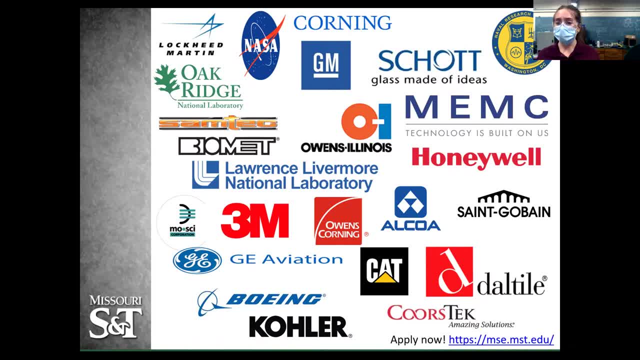 So this slide is full of a bunch of different companies. Everyone needs materials, so ceramic engineers work all over the place. There's a lot of really big names on here. So if you see any of these names up here and you think those are really cool places, ceramics are the place to be, because everyone needs materials. everyone needs ceramics. The starting salary. The starting salary for a ceramic engineering undergrad from S&T is $58,000 to $63,000 a year. So that's just undergrad, no masters. four years in and out, You can be making around $60,000 a year right out of college. 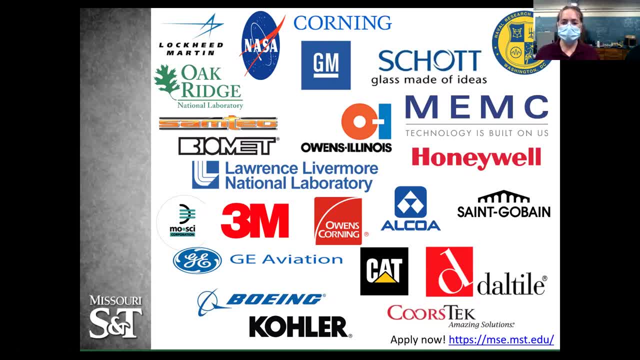 And what's also really nice about ceramics engineering is our department especially. it's about a 50-50 ratio of men to women. So that's really nice, especially because S&T it is a very male dominated campus. Engineering is a very male dominated campus. 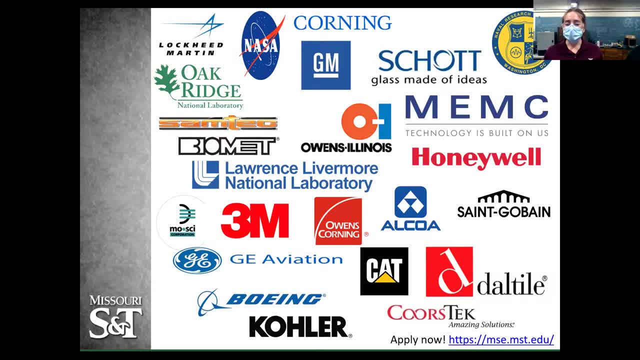 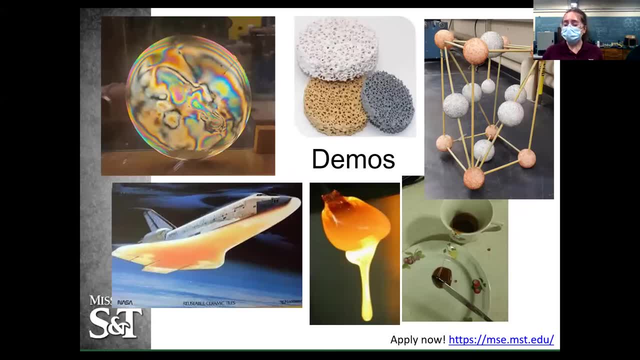 So that's really nice, especially because S&T it is a very male dominated campus. Engineering is a very male dominated campus, So being in a department that has a lot of that diversity is really, really nice. All right, So without any further ado, we'll get into the really fun stuff. 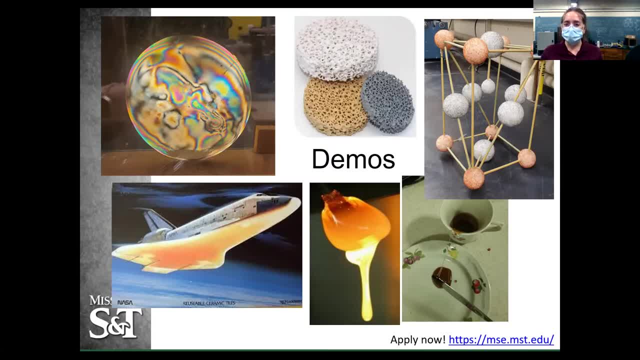 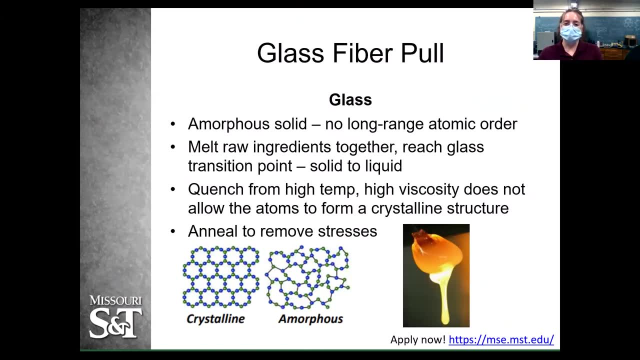 I'll show you guys some cool demonstrations to further explain the cool things ceramics can do. So we're going to start off with a glass fiber pole and I'll just give you guys a brief overview into what glass is. So glass is an amorphous solid. 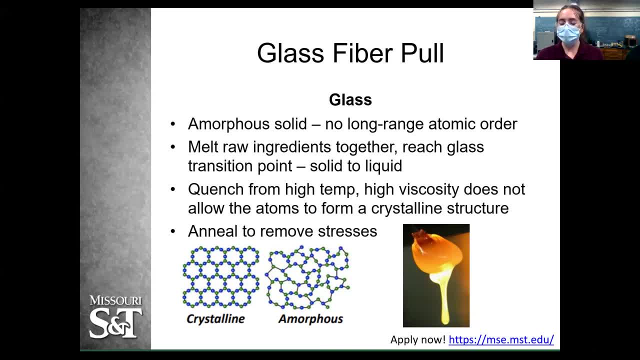 Um, and basically what that means is that there's no long range of mass, Um, and basically what that means is that there's no long range of mass atomic order. So for anything crystalline, you know, if you've got an atom here, you've got an. 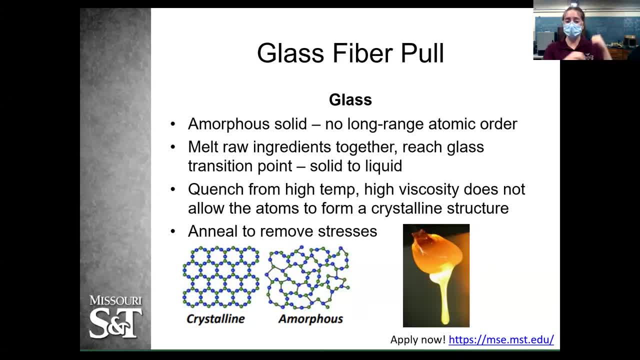 atom. here I can count exactly where all of my atoms are going to be. But in glass that's not the case. If I have an atom here, I maybe have one here, I maybe have one up here, but past that 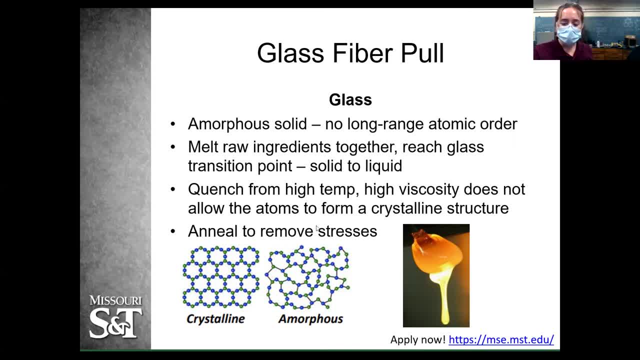 I have no idea where the rest of my atoms are, So you can kind of see down in this figure right here. the crystalline structure is very regular, it's very organized and amorphous, is just all over the place, And that is something that as ceramic engineers we can kind of control to. 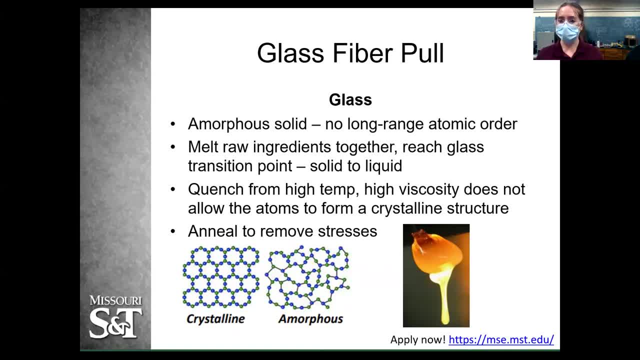 determine where our materials are going to end up and how they perform. This amorphous structure is also the reason why you can see through glass And the way that we make glass is. we take all of our raw ingredients, bring them up to a really high temperature. they get really, really liquidy. 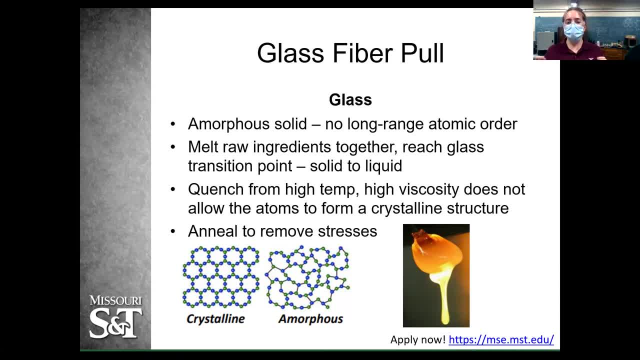 they melt and then they turn into a liquid. And then we take that liquid and we quench it really fast. We take it from a really high temperature down to a really high temperature and then we take it from a really high temperature. 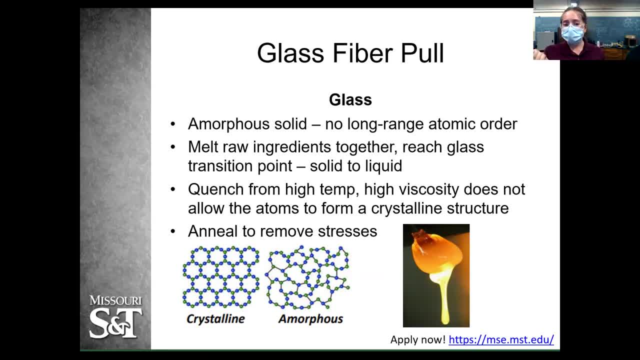 down to a really low temperature like that, And that quenching does not allow your atoms to form together in a crystalline shape. That's what causes them to freeze wherever they're at. So it's like: imagine taking waves in the ocean. immediately freeze all of them. you've still. 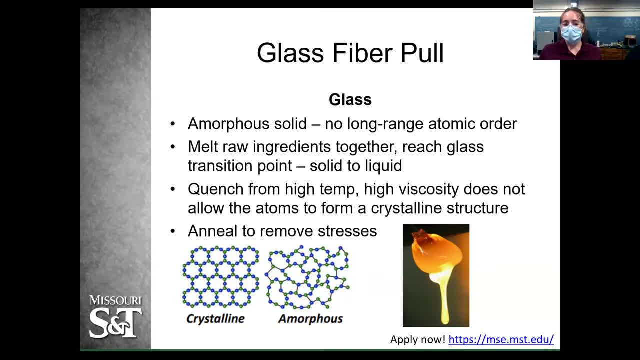 got waves up here, up here, over here, As compared to if you were to slowly cool waves down to freezing, they would even out to a full, to a flat surface. And then, because we do quench, that leaves a lot of residual stresses left over in our glass. 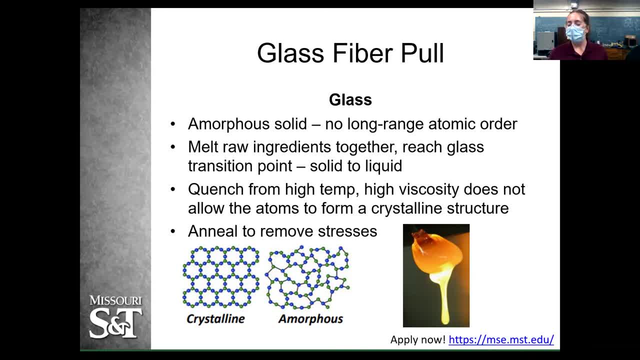 And so we have to do a process called annealing to remove those stresses. And I'll go into that a little bit more in a second and just in our next demo. So we're going to start off, get right into it. We're going to come over here to our furnace. 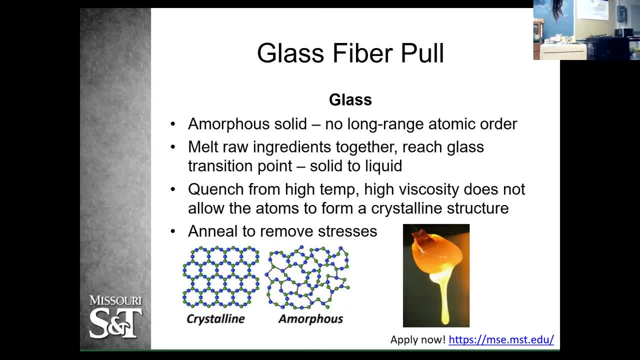 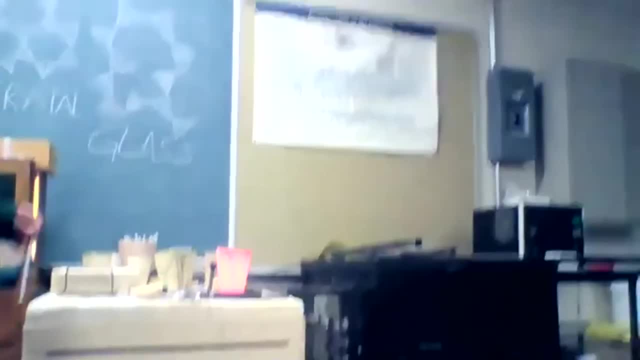 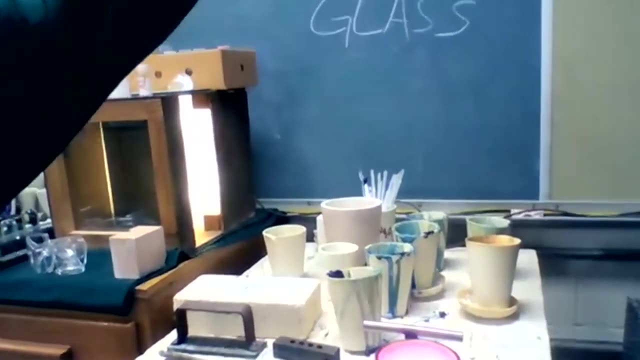 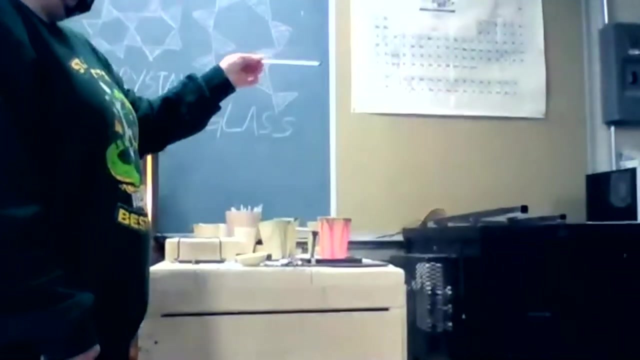 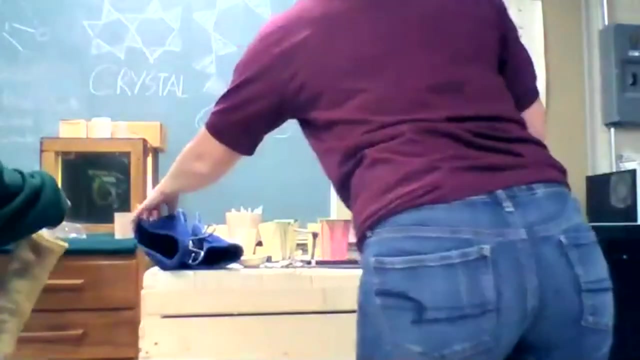 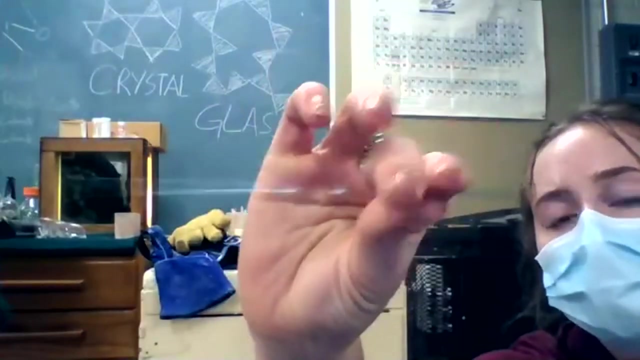 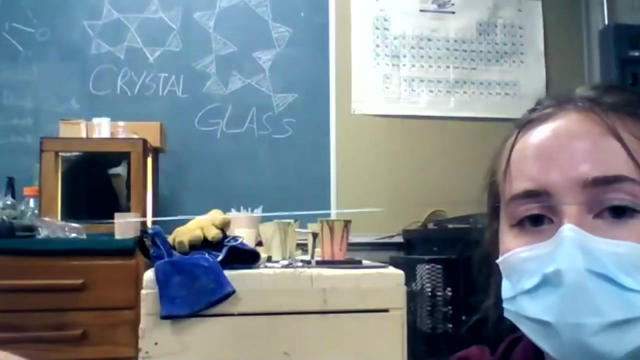 Okay, now I'll set this back down. So now I've got this fiber right here And this, because of its small diameter, has completely cooled, so it's cool to the touch, And this is like. this is how things like fiber optic cables are created, not with this. 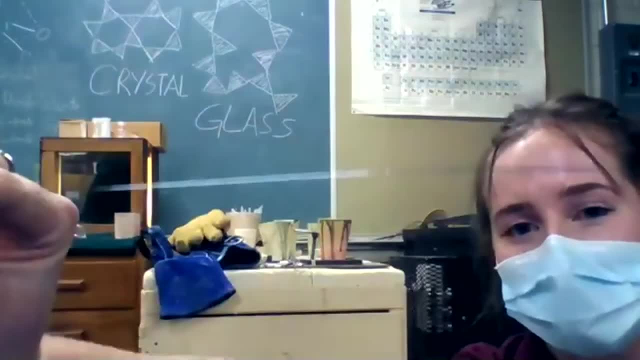 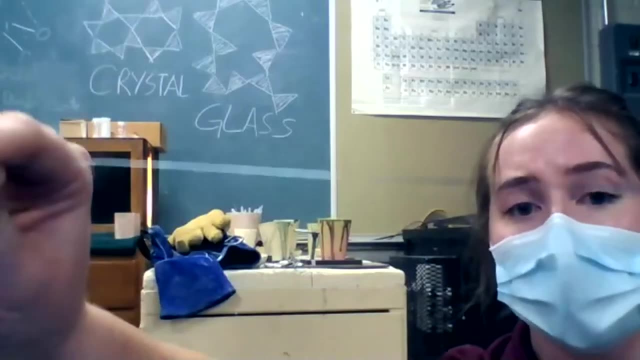 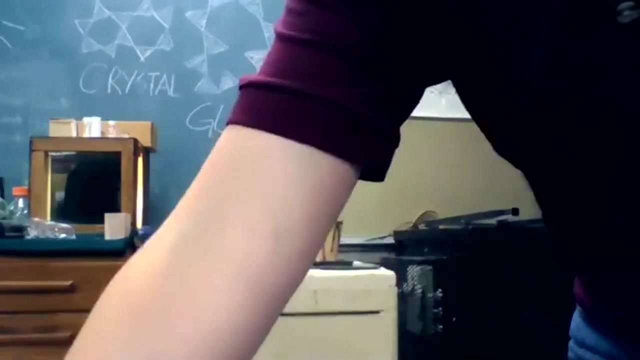 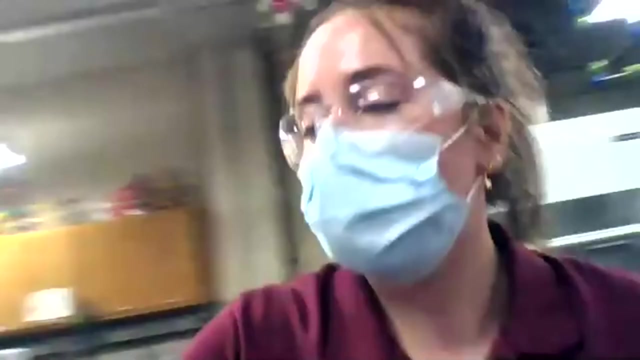 exact process, because it would take a really long time, But this is a glass fiber that we pulled right in our lab right here. So that's one thing. glasses are serenity, so that's something we can do. Okay, So now I'll go into a little bit of applications. 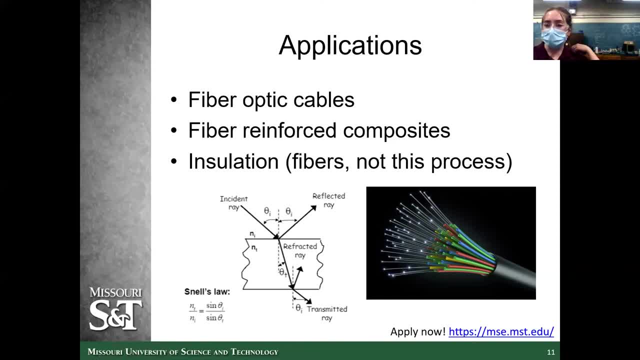 Okay. so, like I said, fibers like that can be used for fiber optic cables, So we can send information down those cables by using a higher index of refraction on the outside of the glass and a lower index of refraction on the inside. 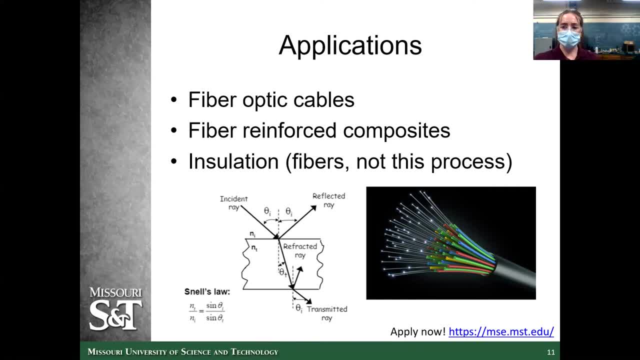 And that way the larger the glass the better. So that way the light bounces back and forth between the fiber all the way down the length of the fiber to send that information. So things like Google fiber uses fiber optic cables. they're all over the place. 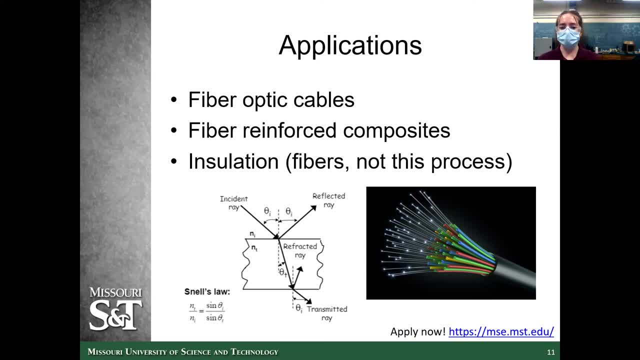 They can also be used in fiber reinforced composites. So that's just a mix of several different materials, And the fibers in the composite make the material much, much stronger, because cracks can't make their way through the fiber. Okay, So that's just a mix of several different materials that can make their way through the fiber as easily as they can through a solid material. 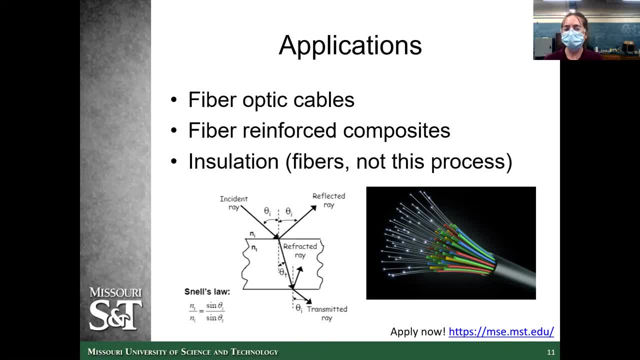 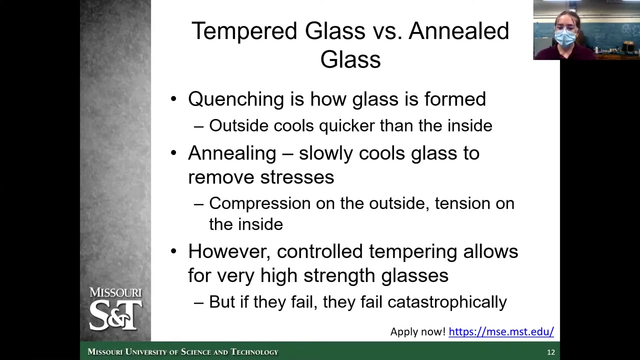 Things like fiberglass insulation also uses fibers. not this exact process, not pulling fibers like I just showed. It's more like when you think of cotton candy being formed. that's how fiberglass insulation is created. Okay, So now we'll go into another glass demo. 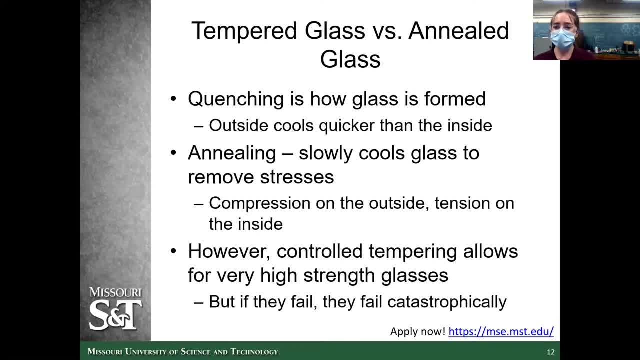 So, like I said just a little while ago, the stresses in glass have to be annealed out to prevent catastrophic failure. So, like I said, quenching is how glass is formed. but when we do that, the outside of the glass cools much, much faster than the inside. 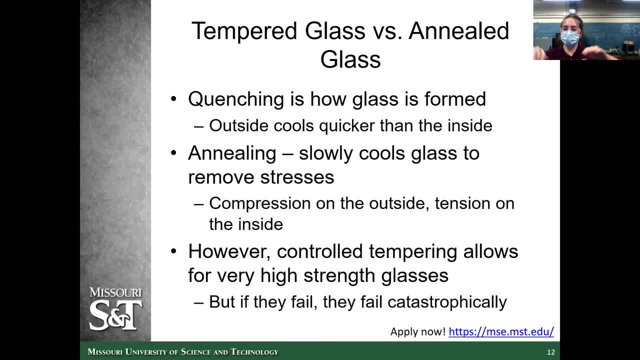 So if you have a big blob of glass and you quench it really fast, the outside freezes in place immediately, but the inside still has a lot of heat- It's still really warm inside there- And so when that happens, The glass on the outside goes into a compression stress, but the glass on the inside goes into 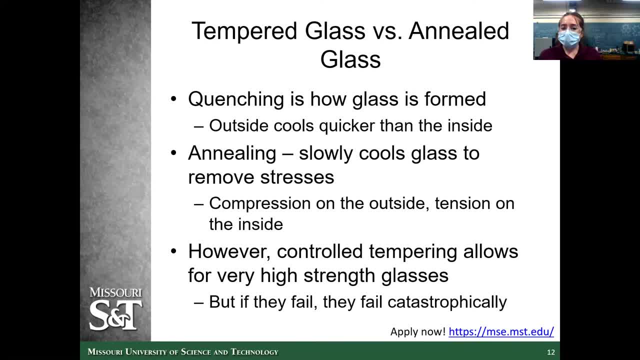 a tension stress And so if we don't take care of that, it can. it basically looks like it blows up, It breaks at the speed of sound. It goes really fast. So it can be super dangerous if we don't take care of those stresses. 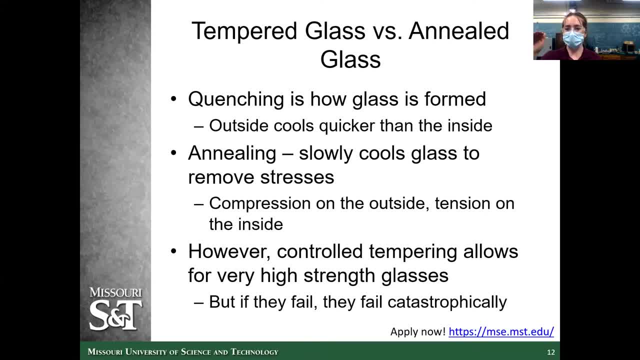 And again, we do that through a process called annealing, which is just taking the glass from a high temperature and very, very slowly cooling it down to room temperature. However, If we do a controlled tempering, we can allow for a really really high strength glass. 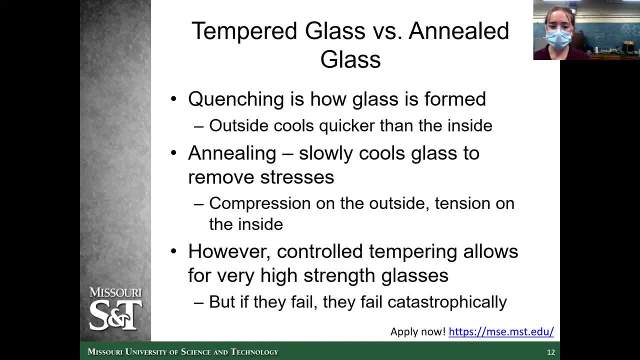 And so now we'll kind of demonstrate what those stresses look like and what that means in an application. So we'll come over here. This is a polarizer. We've got two panes of glass and they're polarized in opposite directions so that the light that 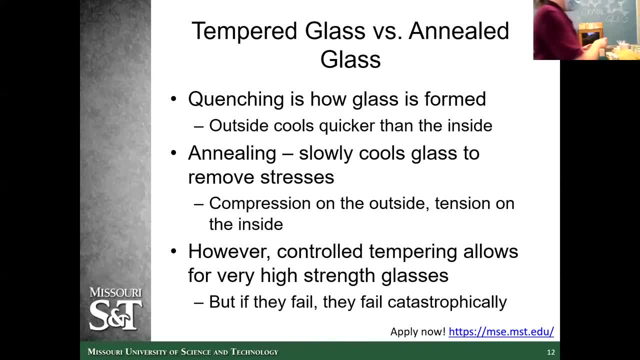 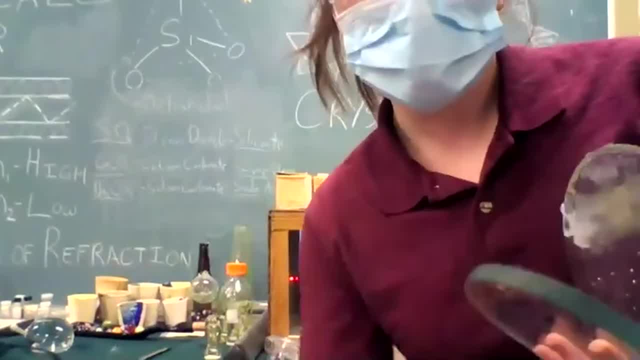 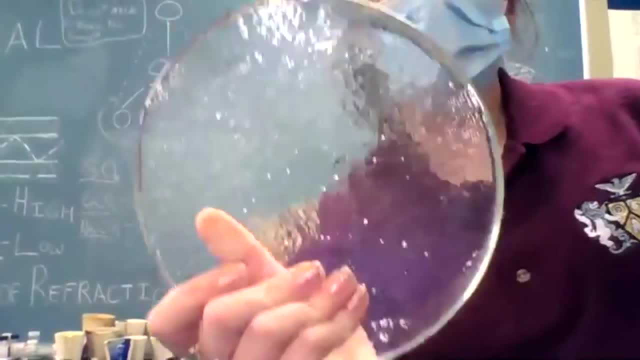 shines through is only coming out in one direction, And so we can see this. This is a polarizer. This piece of glass is annealed, so there's no stresses. So there's no stresses in this glass, But this glass has been tempered. 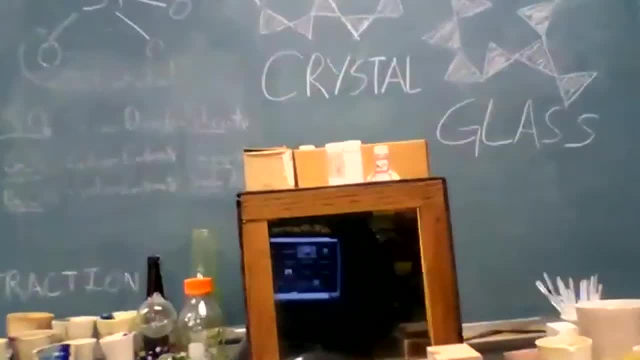 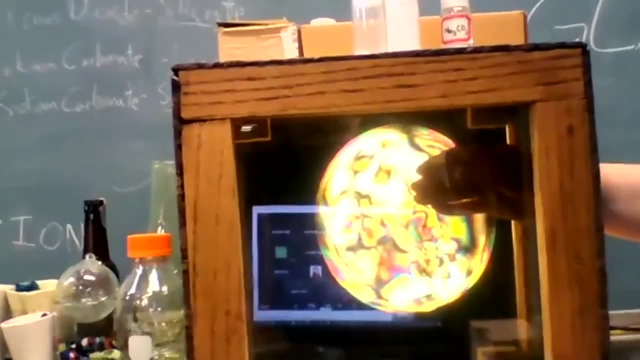 So there's a lot of stresses in this glass, So Can you get up really close? So if I shine this through here, you guys see that there's like a rainbow of colors And those colors antiphase, with stresses left in that piece of glass. 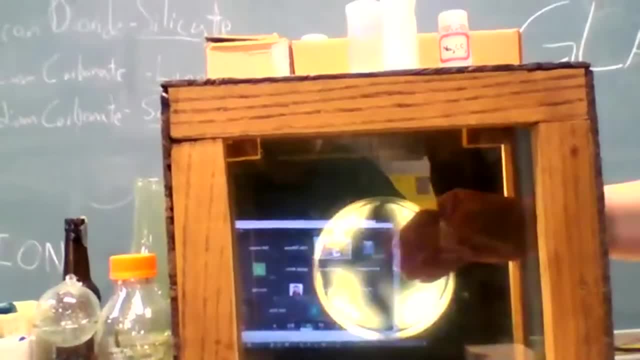 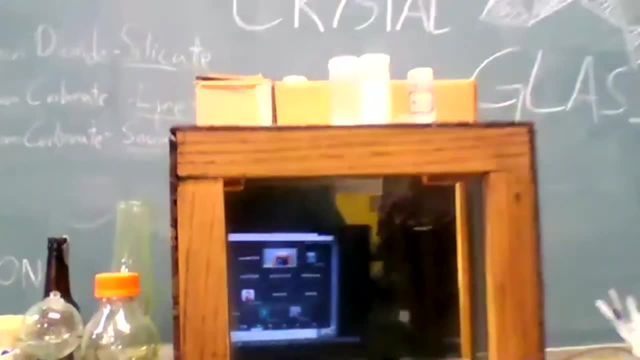 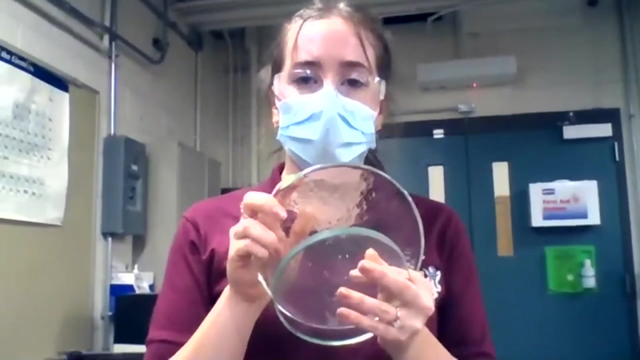 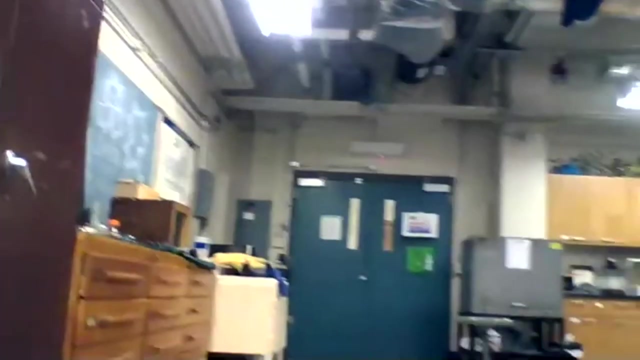 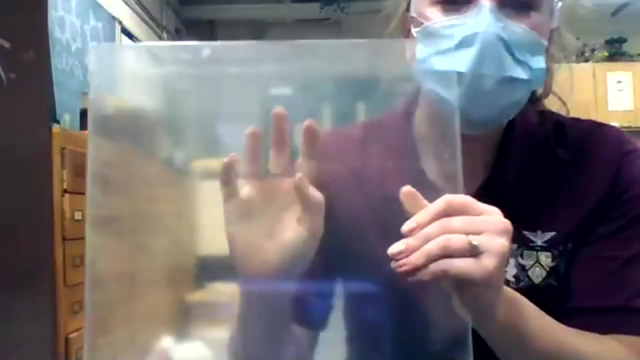 glass. But if I do a new glass, it's more gray. So again, if we break the compressor or the compression layer on the outside of this glass, it'll break immediately, And so we'll demonstrate that. So this piece of glass is tempered, And just by looking at it you 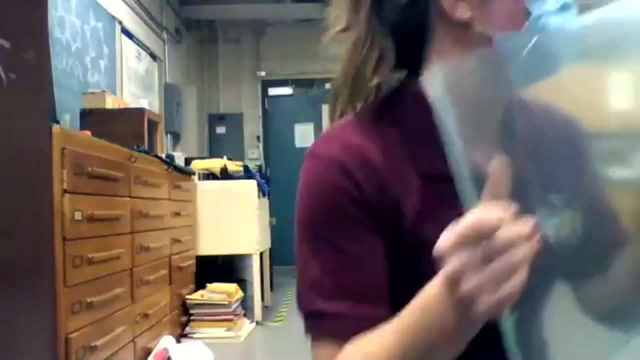 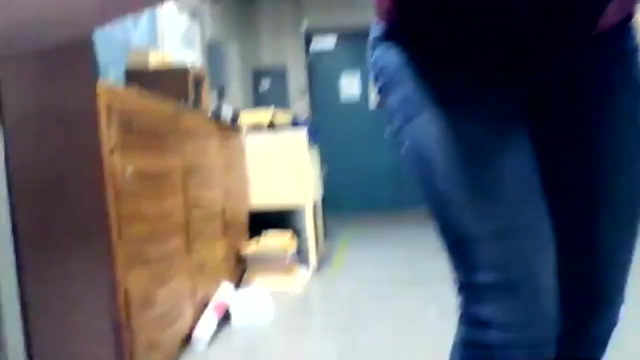 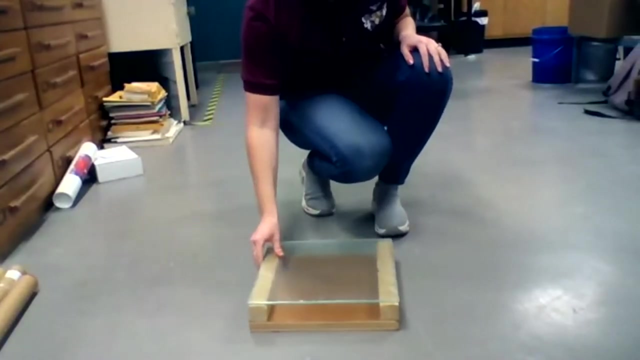 would never be able to tell, But I'm going to show you guys how we can tell. So I'm going to set this glass on the ground. So, like I said, tempered glass is really, really, really high strength. So I'm going to go ahead, I'm going to stand on this glass, I stomp on it, I jump on the. 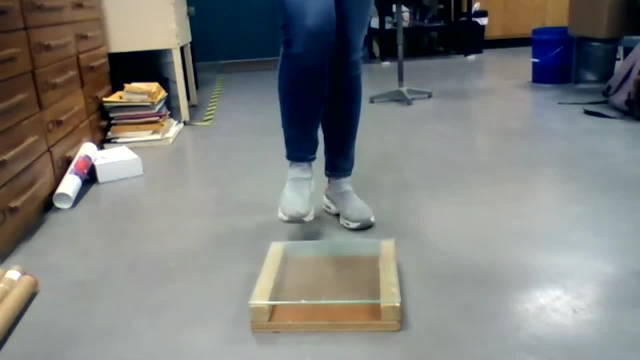 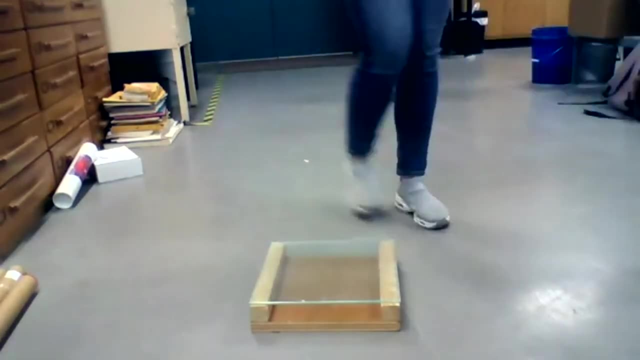 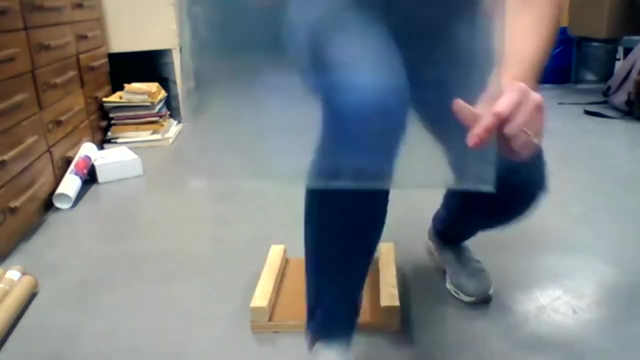 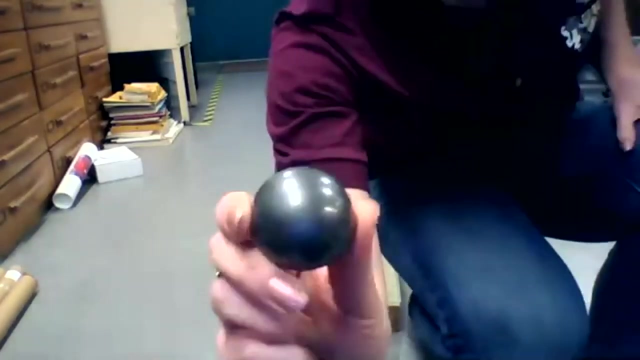 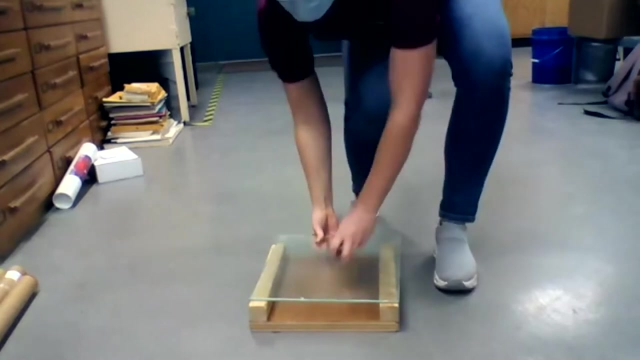 down on it, It's not breaking, It's not going anywhere. I can even take this metal ball and I can drop it And my glass is still intact. But let's try this even bigger ball And again my glass is still completely intact. 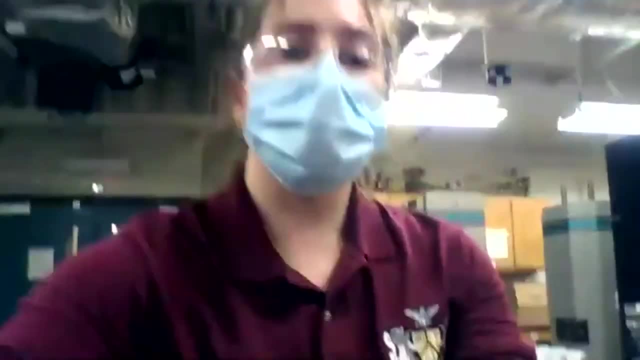 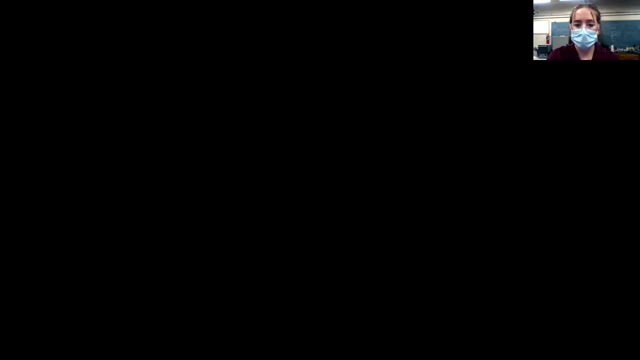 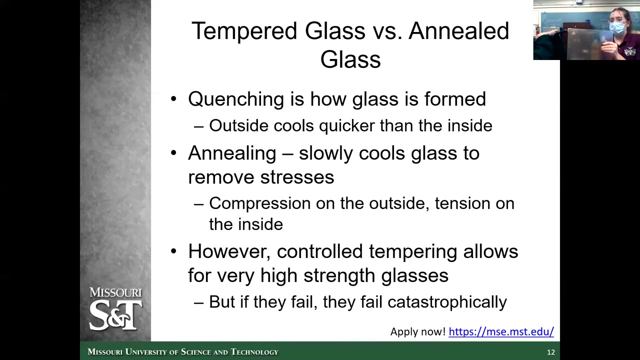 However, like I said, if we can break that compression layer on the outside, we can show that this glass is tempered. So we're going to try this even bigger ball breakage pattern. So Sophie's going to take my snippers right here and she's just going to go. 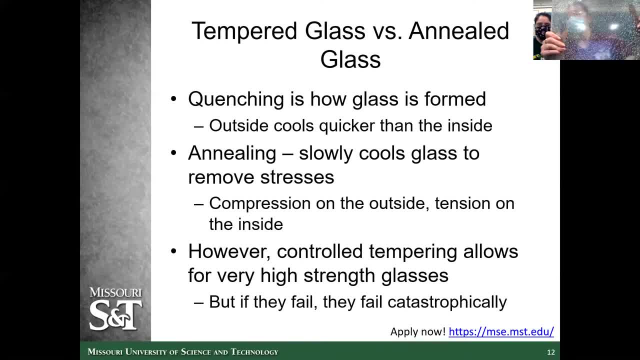 in on that corner, And now we can see those tension forces on the inside spread out at the speed of sound to relieve those stresses inside the glass. And so this is what tempered glass when it's broken. this is what it looks like. This is annealed glass, So you can see the annealed 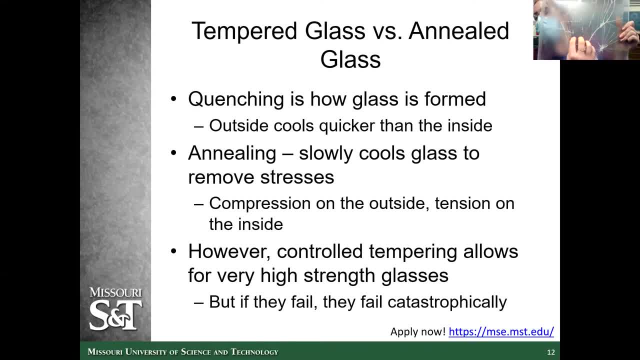 glass the stresses weren't nearly as high. so we get this spiderweb kind of cracking pattern. But again with the tempered glass it just blows into a bunch of bunch of different pieces, And so applications for this tempered glass includes carved windows and phone screens. 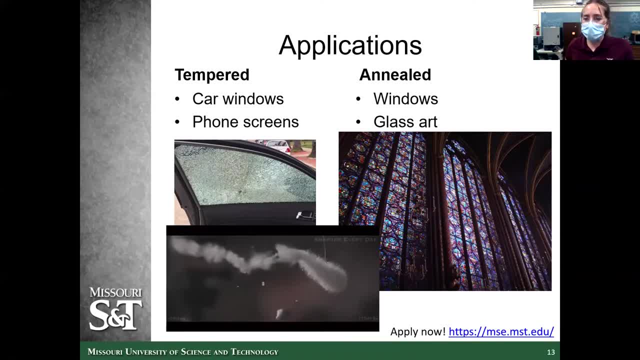 for the annealed glass. There are things like window panes and glass art, So like when I was talking about the Gaffer's Guild earlier. all of those pieces have been annealed so that if they break they don't burst into a million pieces, And this gif on the bottom right here shows a Prince Rupert's drop. 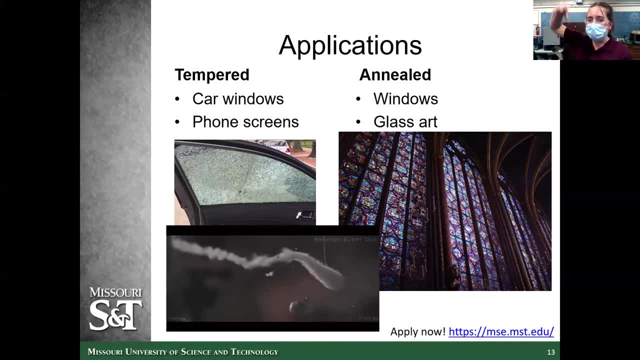 And that's just a piece of molten glass that's been dropped into a bucket of water And, like I said, it immediately quenches it into a solid. And this bulb on the end is super, super high strength. If you see right in here, that's a bullet. Someone shot a gun. 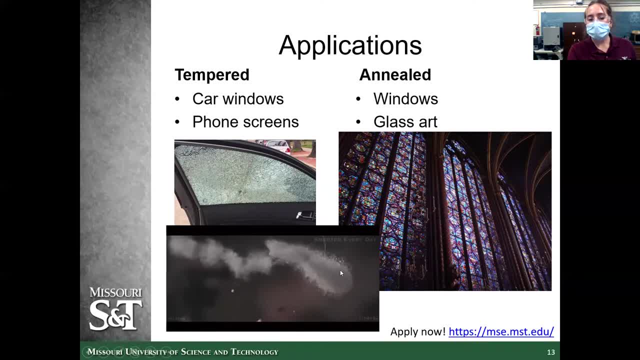 at this Prince Rupert's drop, And the reason it shatters is because the tail, which is really thin up here, vibrated enough that it snapped and then it broke all the way down. So even with the force of a bullet, the Prince Rupert's drop will not break. So tempered glass is very. 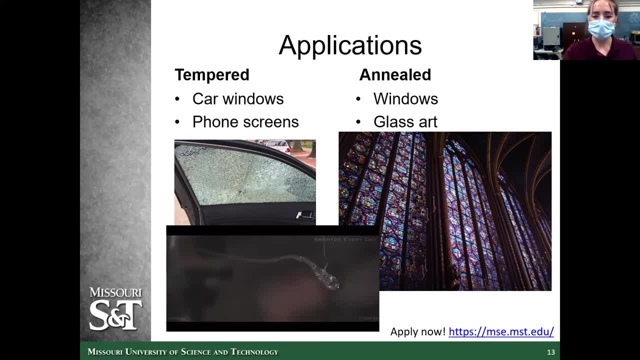 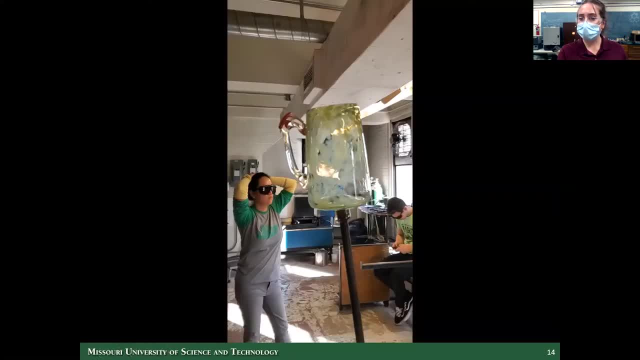 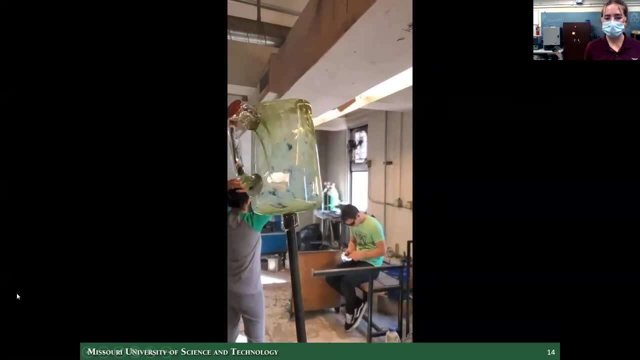 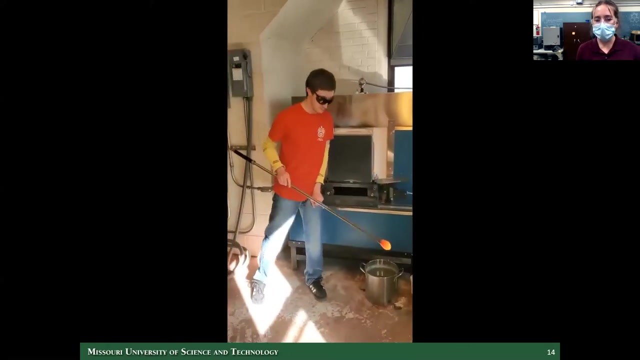 very high strength and it can be used in a lot of really cool applications. So this is just a short video to show what our Gaffer's Guild, what our hot glass shop, can do on campus. So this was two years ago now. They were making a mug to sell in the St Pat's sale. 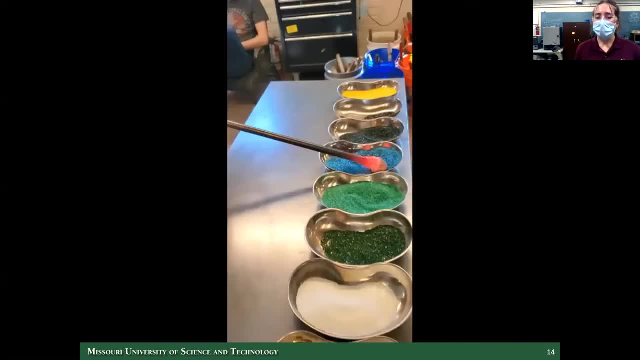 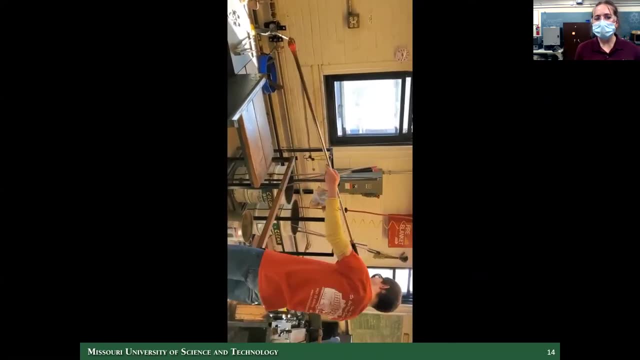 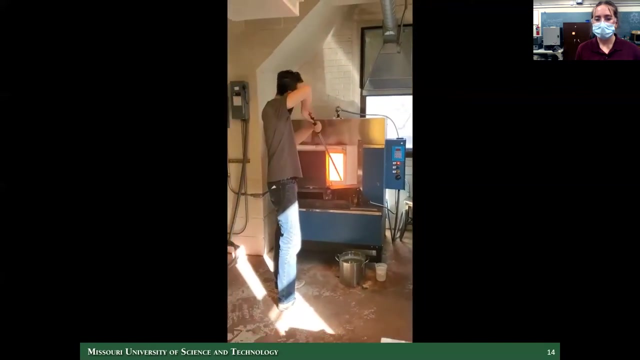 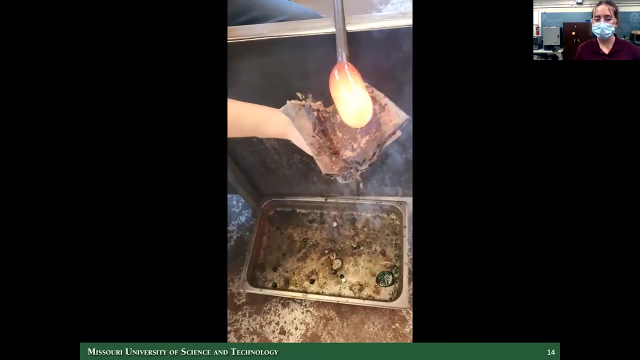 So the Gaffer's Guild is completely student run, student led. All the proceeds that they make from selling their glass pieces go right back into the shop so that they can keep it running and keep doing really cool, really cool stuff. You can see by using that- the heat in the glass. 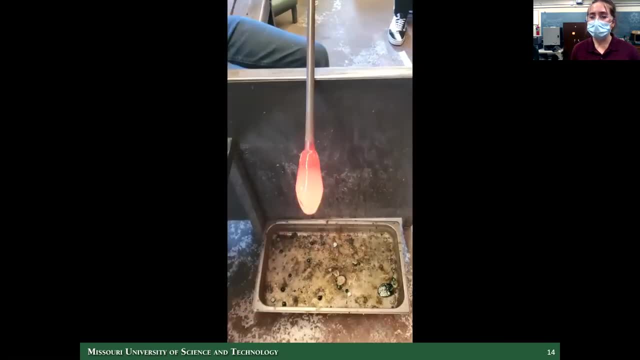 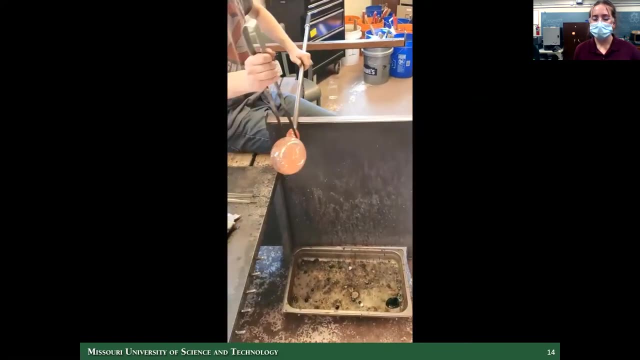 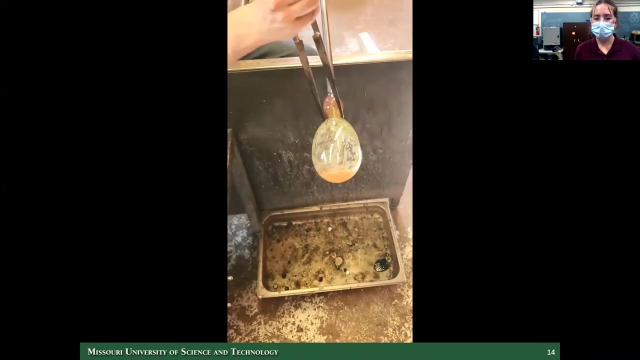 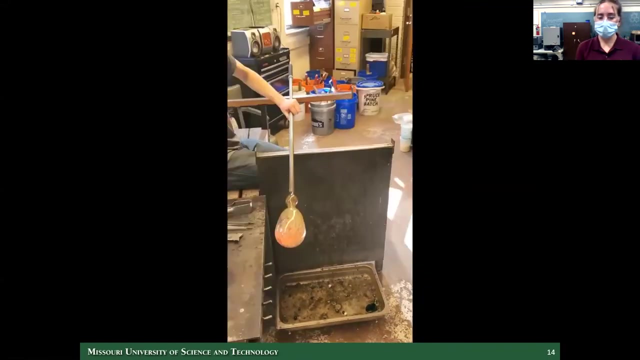 he's able to control that, to form the glass in whatever shape he wants. So the the the name of the wine is the St Pat's. it's pretty simple. But the other issue that he was told about was that, you know, this is a giant glass and he has to make it bigger. 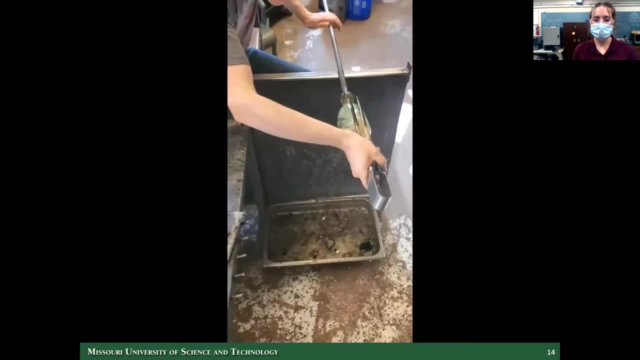 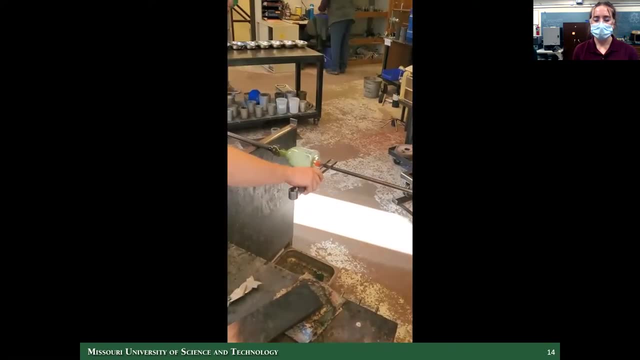 So he's one of those people that's able to make it step up here And in the in the shop. you know she wanted it to be so big And you know she's able to make it fit Yeah. 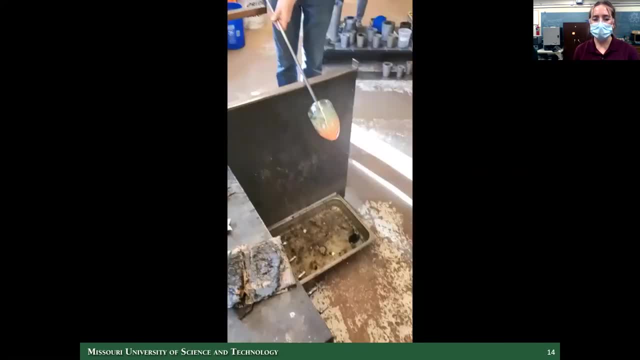 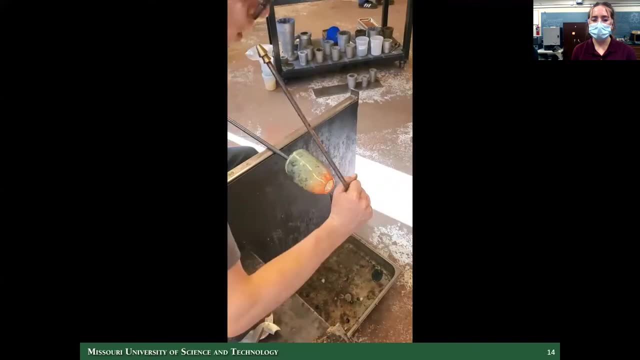 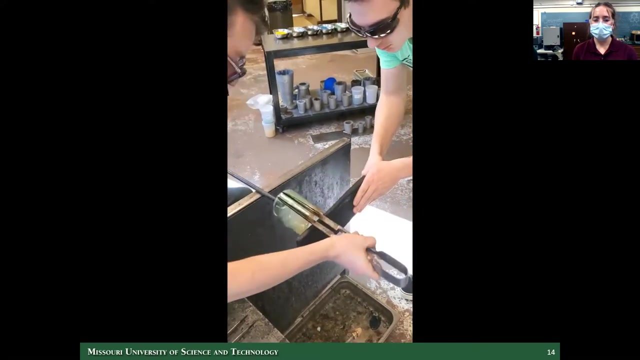 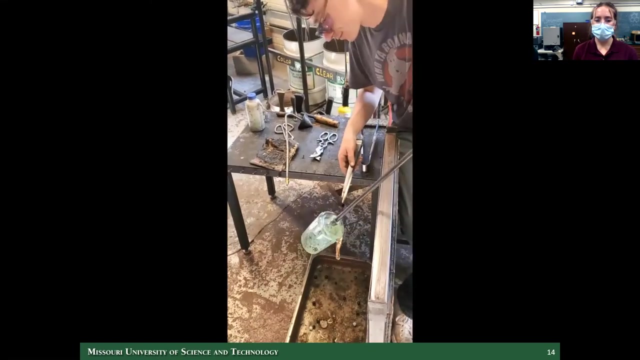 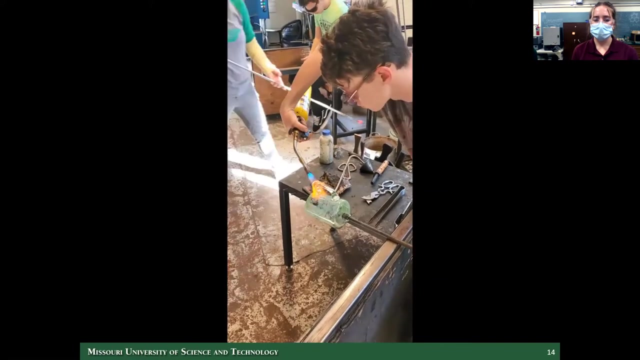 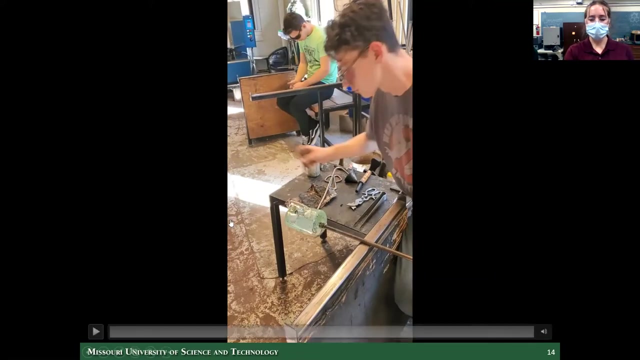 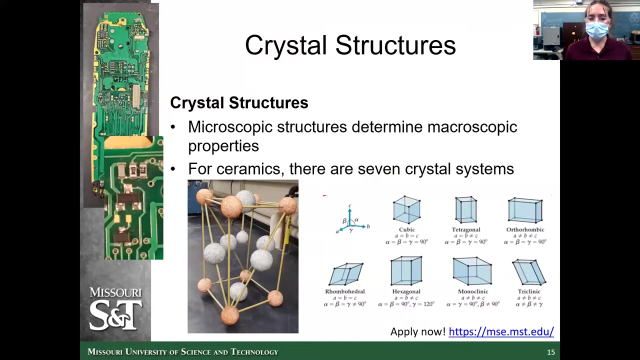 So look at that, Yeah Yeah, the blowpipe to work on the opening of the mug, And there's the finished project. So now I'm going to talk a little bit about crystal structures. So, like I said at the very beginning, ceramic engineers and material science engineers manipulate the microstructures of materials to determine the macroscopic properties. 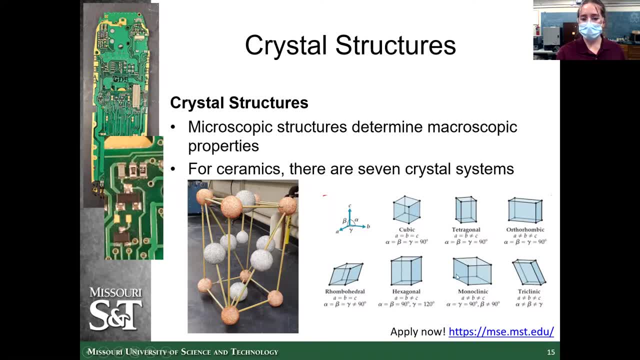 For ceramics. there are seven crystal systems demonstrated here in the corner of my screen, And by using those crystal systems and using different materials that exhibit different structures, we can make really cool materials out of them. So this structure I have right here, I also have it on my screen right here. 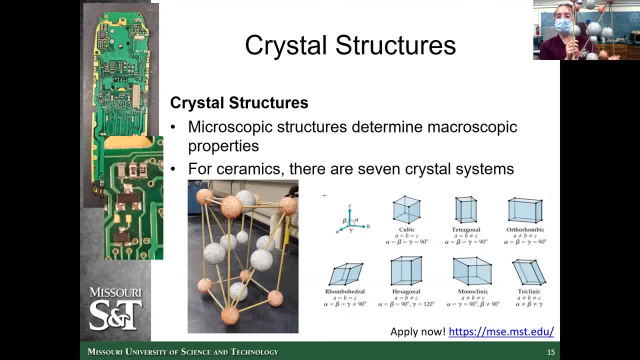 This is barium titanate. So this is a really cool material because, if you can see, in the center here there's a very small atom. This is the titanium atom, right in the center. When you push on this structure, you put this titanium atom out of where it usually is. 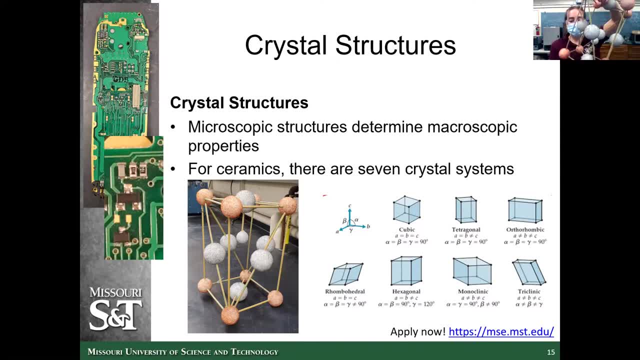 And by doing that you create an electrical current. So basically what that means is, when you push, when you put a mechanical input into a barium titanate structure, you get an electrical output, So that can be used in all sorts of ways. 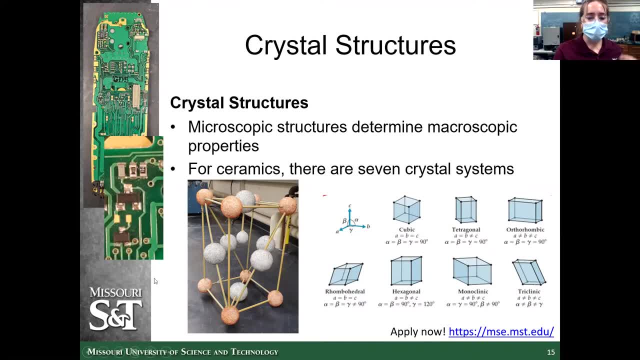 They're used in capacitors. So these pictures I have over here, these are capacitors in cell phones. They're everywhere. There's really cool things. I've seen stuff like if you guys have heard of the military using battery packs on their shoes to power electrical things while they walk. 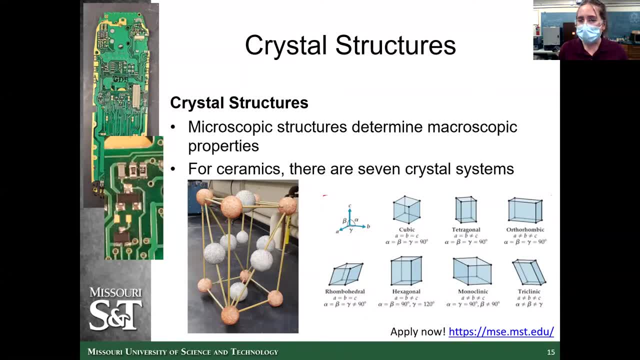 That's because of perovskite structures they're called Those materials- that when you put the mechanical force on them they create an electrical current. So you can harvest that electrical current and use it in a bunch of different ways to create different really cool materials. 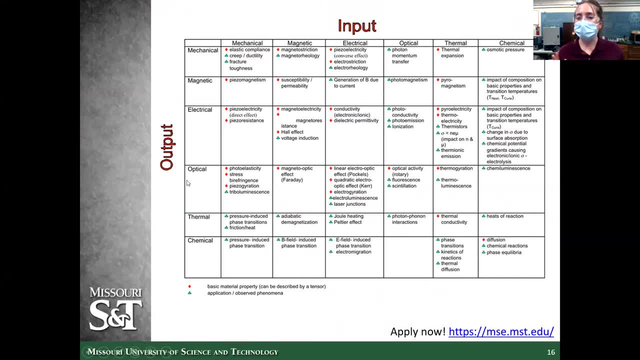 And so this table, what you see right here- this is something we see all the time as a ceramic engineer. Up here is all my inputs. So the one I was just talking about is a mechanical input and the electrical output. It's called piezoelectricity, where you put the mechanical force on it and you get an electrical current. 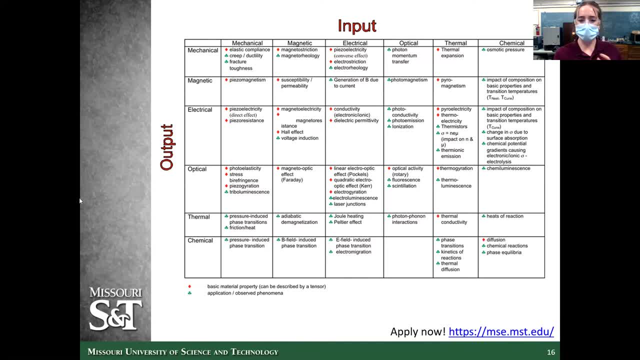 But other than that, all of these have some sort of ceramic material that go along with them. So ceramics can be used all over the place, not just in toilets. So ceramics can be used all over the place, not just in toilets. So ceramics can be used all over the place, not just in toilets. 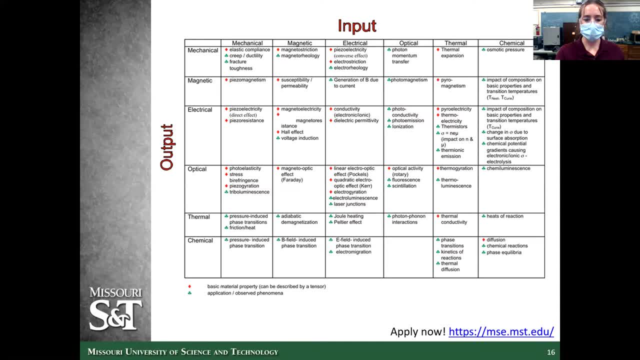 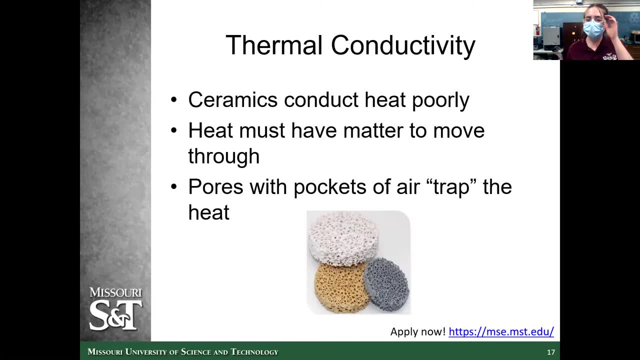 Or glasses. they can be used everywhere. So next I'm going to talk to you guys about thermal conductivity. Like I said at the very beginning, ceramics are really good at heat. They conduct heat poorly. They're very heat resistant. Heat must have matter to move through. 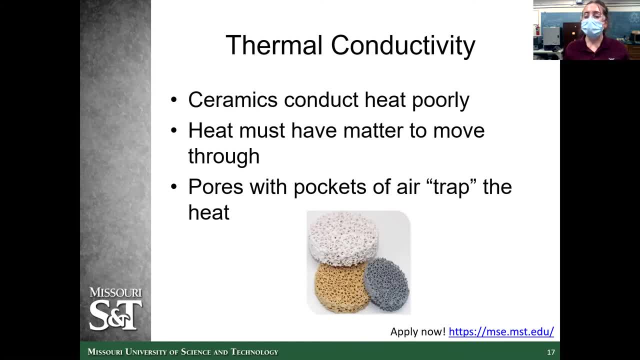 And when it doesn't have matter to move through, it just stops. And ceramics are very porous So they have lots of air trapped inside themselves. So you can see these pictures I have down here. The ceramics have all these pores so heat cannot travel very well through there because there's no way, there's nowhere- for it to get from point A to point B. 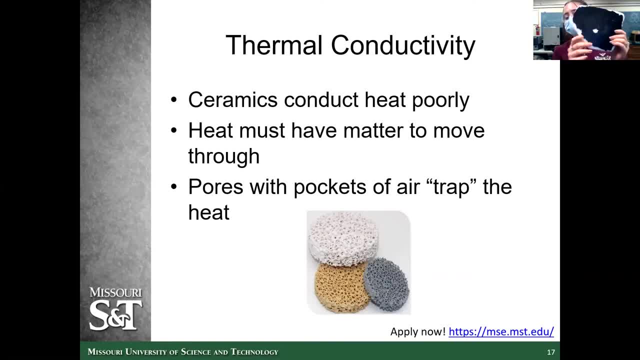 So we're going to demonstrate this one. This is a space shuttle tile, So this is what they line the outside of a space shuttle with to protect it from the heat from entering the atmosphere. So this protects the astronauts and all the electrical equipment from burning up in the atmosphere. 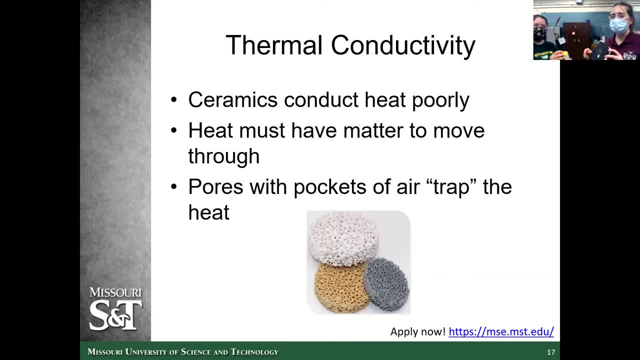 So we're going to show. We've got a torch right here And I'm going to heat this side up right here And you can see now this is red hot, But I can touch the back of it, no problem, It's completely cool on the other side. 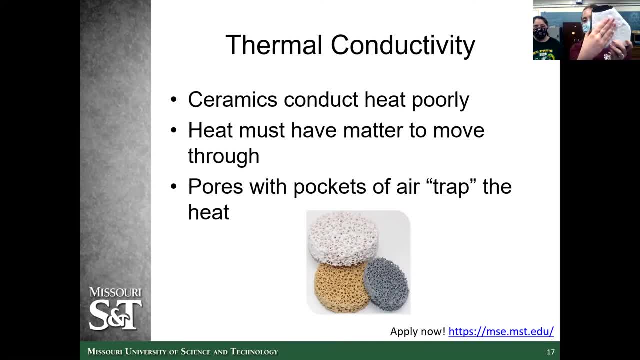 There's no heat passing through this material to keep my hands safe on this side. So something this thin traps the heat so well that I don't get burned on the other side. And that was red hot. It was blowing red hot And then obviously you can see it dissipated very, very quickly. 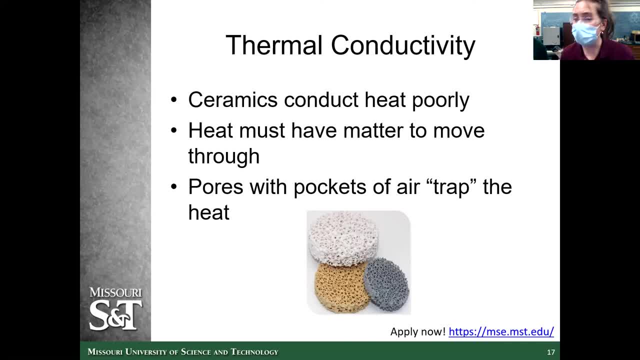 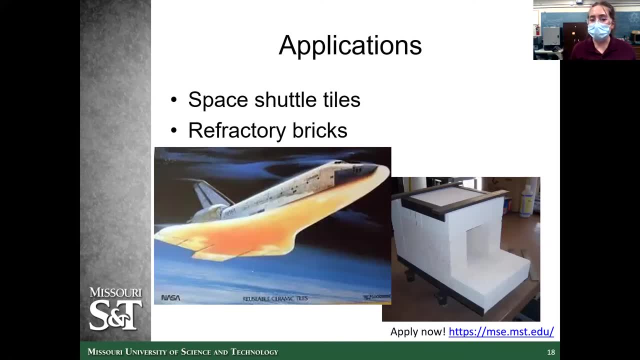 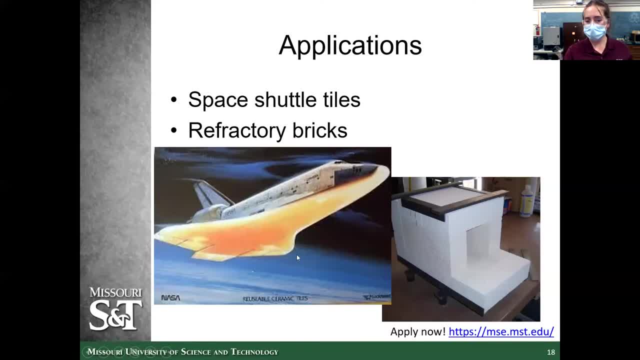 So right here, these would be all ceramics. This is exactly what I just showed you. They're aligning that space shuttle to prevent it from burning up in the atmosphere. We also use them for refractory bricks, So those are things that line outside of a furnace to keep the heat in. 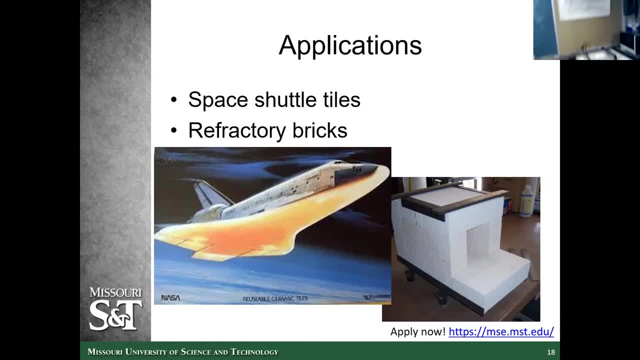 Like I showed earlier with the fiber pool, this is our furnace That's at 1,100 degrees. Surrounding that is ceramic. Those are refractories, so they keep the heat in and they're also very, very resistant to the heat. 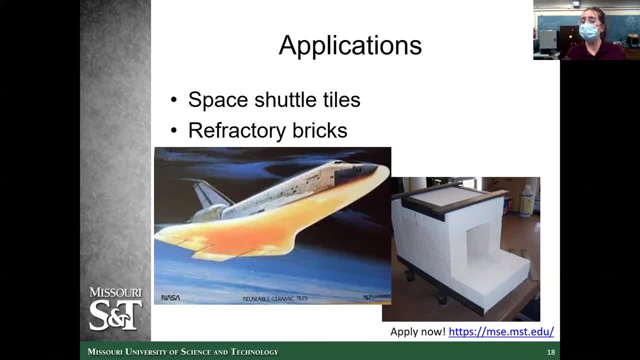 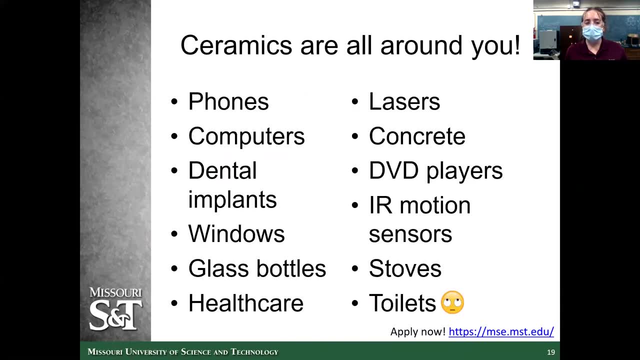 So we can use them over and over and over again without them burning up or melting or anything. So ceramics are all around you. I hope after this little presentation I hope you can kind of see that more now. Like I showed, they're in your phones. 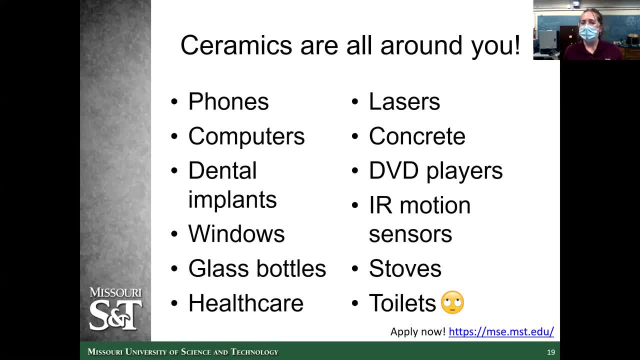 Those electrical ceramics are all over the place. They use them in computers, dental implants. They're very chemically resistant so they're safe for body use. Windows, like I showed, glass bottles, lasers, concrete DVD players, iron motion sensors. 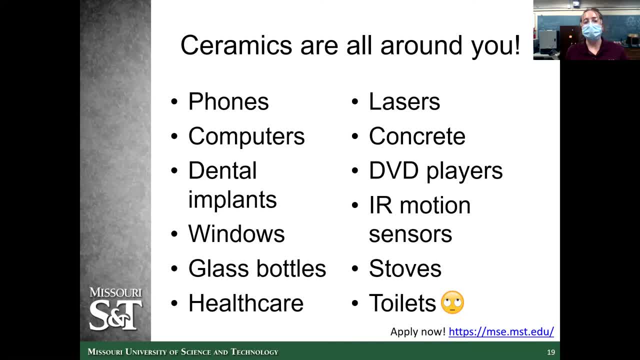 stoves and, yes, toilets, But ceramics are everywhere. They're a very, very cool material. There's lots you can do with it. You pick a field you want to go into. You can go into it with ceramics. So ceramics are utilized in everyday life, even if you guys don't realize it, kind of. 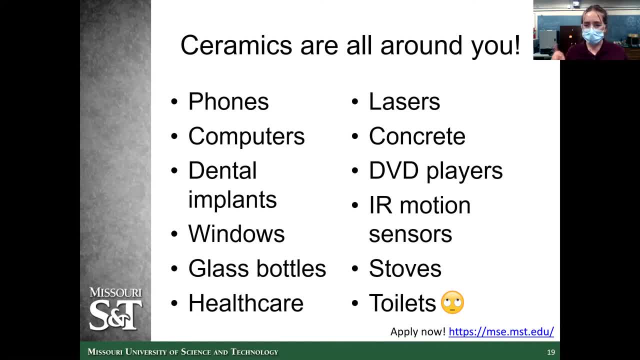 like I just said, And there's advanced versus traditional ceramics. So I talked a lot about the advanced ceramics today, but there are a lot of traditional ceramics. That's something that we're going to talk about in a little bit, And then we're going to talk a little bit about the traditional ceramics. 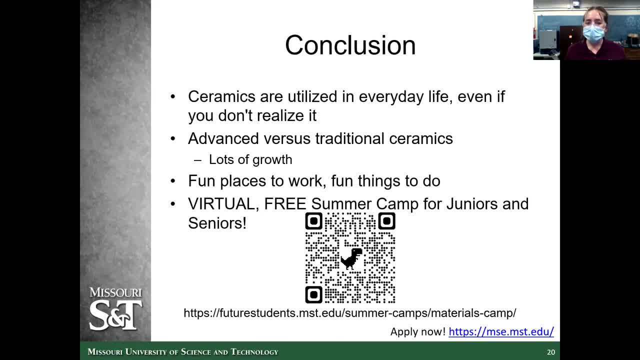 And then we're going to talk a little bit about the traditional ceramics. And then we're going to talk a little bit about the traditional ceramics. So there's lots of things like the refractory bricks and stuff, but there's lots of growth to be done in ceramics. 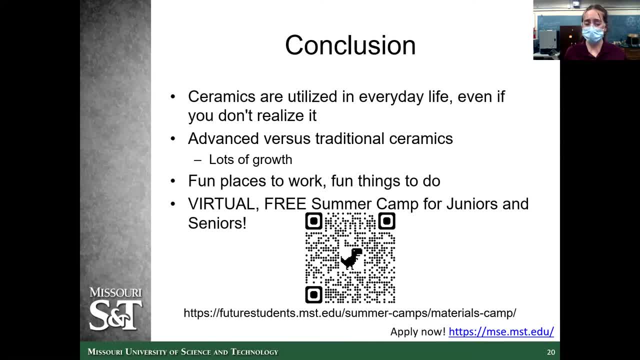 If you guys are interested in going to a field where there's lots of things to discover and lots of growth to be had, ceramics is a really great place to do it, because they're on the cutting edge. Advanced ceramics are on the cutting edge of technology right now. 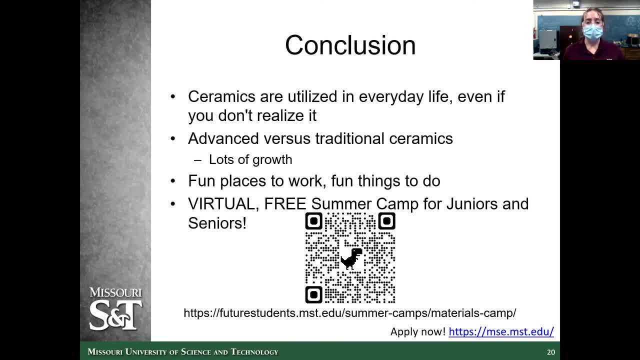 There's fields everywhere to go into And, like I said, there's fun places to go. There's really big names: NASA, Tesla, SpaceX. There's a lot of products. There's a lot of electronics all over the place There's you can go anywhere with ceramics, Um, and there's lots of fun things. 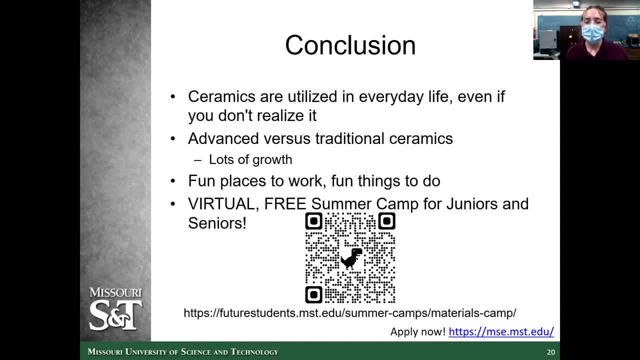 to do And right here at the bottom I have a QR code. Um, we have a free summer camp this summer and it is virtual so you can do it from anywhere. um, for juniors and seniors. So if you guys are, 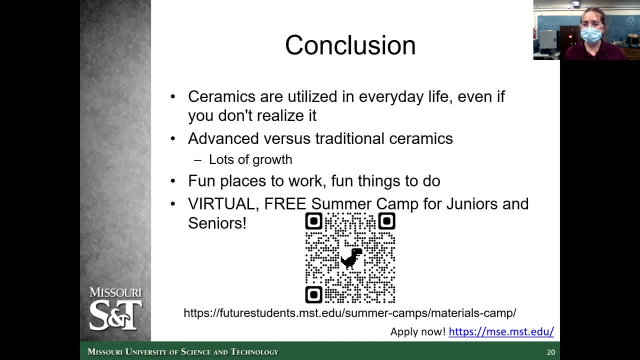 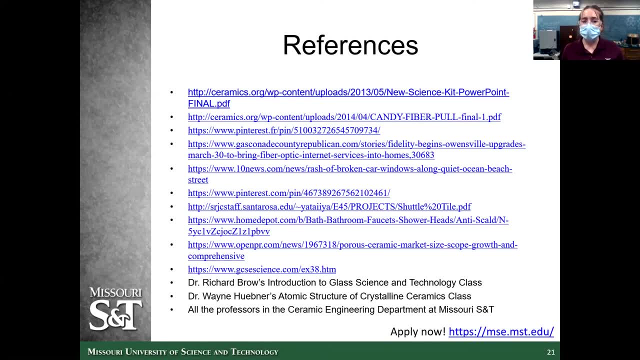 interested in that? um, go ahead and go to that link, go to that QR code and check it out. Um. and then my last page just has a couple extra resources. If you guys are really interested in this, check any of these out there. They've got really good information and really good. 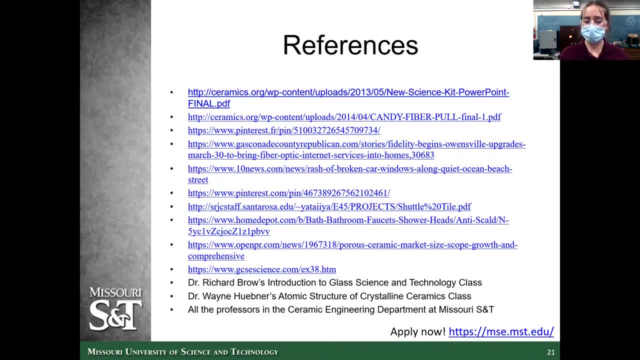 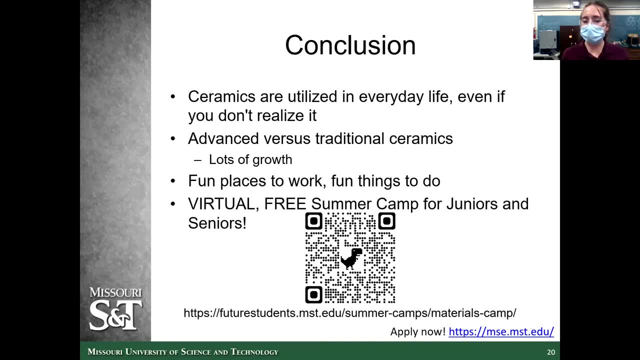 um diagrams and more demonstrations to show. So with that I think I'm done. Um, if anyone has any questions, I'll open it up now. Please just type your question in the chat and we'll answer Claire. so a question that I'll start off with just to get things going, would. 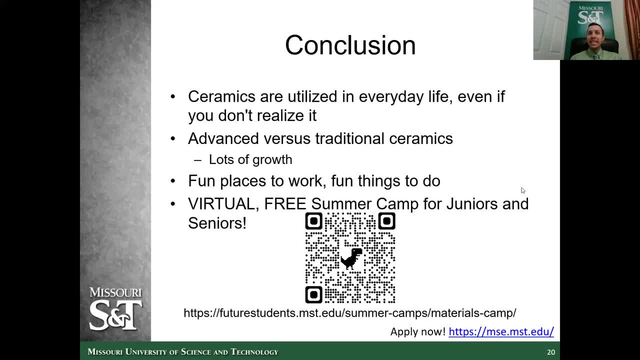 be um. what are some of the most important things that you've done in your career? Could you answer why you chose Missouri S&T and then related why you chose specifically ceramic engineering? Absolutely, Absolutely So. I grew up in Kansas City, Missouri, so I'm only about. 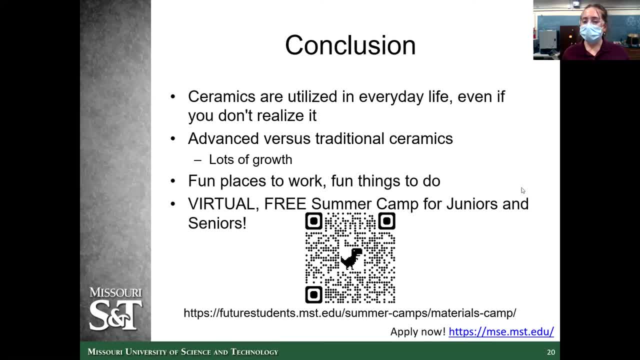 three hours outside of Rolla. Um, and in high school I really really enjoyed my science and my math classes, So engineering seemed like the way to go. Um, and then I visited S&T and decided I really liked the campus. I really liked the buildings, I liked the atmosphere. Um. 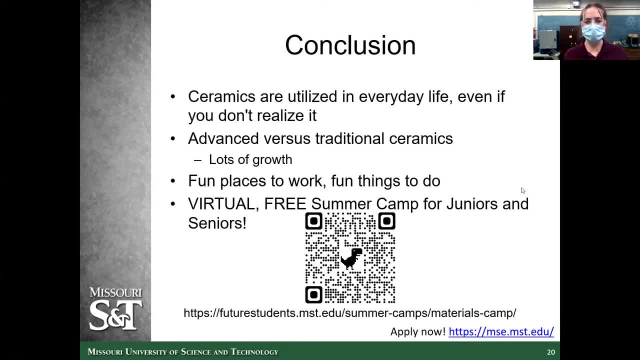 so that's why I decided on S&T For ceramics. I actually didn't come into S&T as a ceramic engineer. I started off as a chemical engineer. um, because I, like I said, I really, really liked chemistry in high school. So I was thinking, oh, I really like chemistry. Obviously I need to go to. 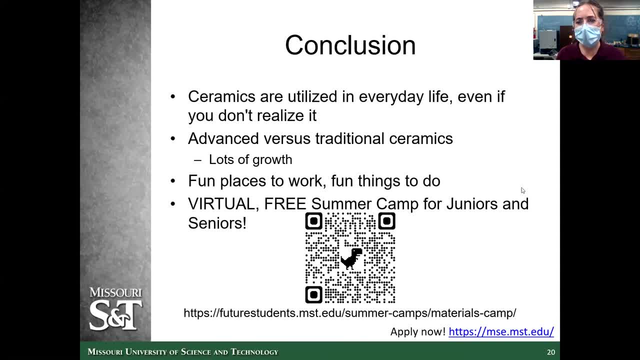 chemical engineering. And it turns out chemical engineers don't actually do much fun chemistry. It's the ceramics that do the fun chemistry. So that's what drove me into ceramics and why I ended up where I'm at. Uh no, So I did not tour any other engineering schools. Um, I came to S&T and I fell in love with 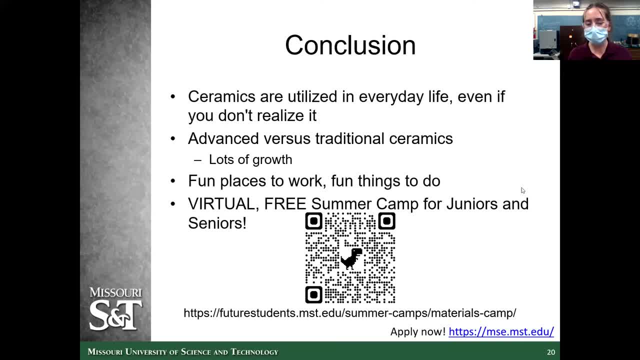 it immediately. Like I said, I really, really enjoyed the campus. I liked the location, I liked the buildings um and everything it had to offer. There's ceramics are only offered at, I think, two colleges, Two, four, Yeah. 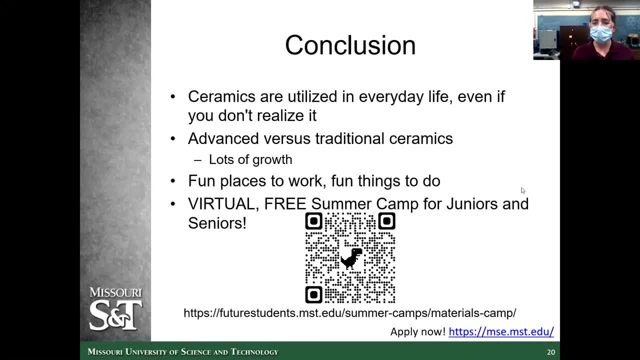 For undergraduates, ceramics are only offered um at two universities in the nation. So if you guys are interested in ceramics, you're really limited on options. but S&T is a really great place to come. We've got really great professors and really great atmosphere. 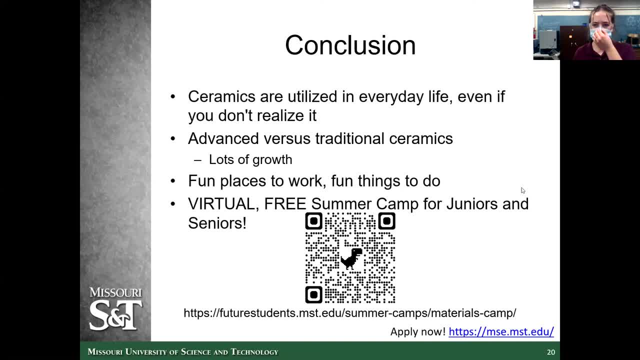 So I don't have anything else. I know I went kind of fast through that. If you've got any questions or if I breezed over something, if you're confused about anything, please feel free to let me know. I can go back over anything. 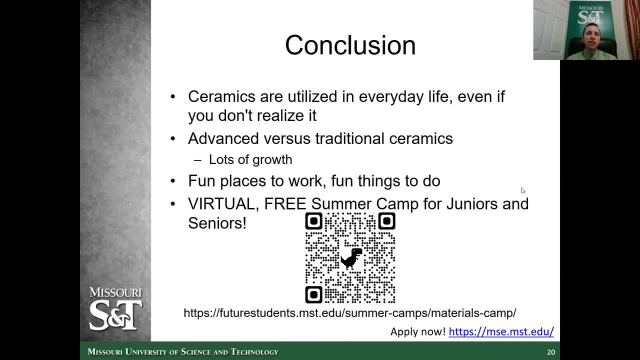 So the next question we've got for you then, Claire, is: can you talk about in high school, uh, what were your favorite science class may have been Yeah, Yeah. So I took chemistry my sophomore year of high school. Um, I knew I liked science. 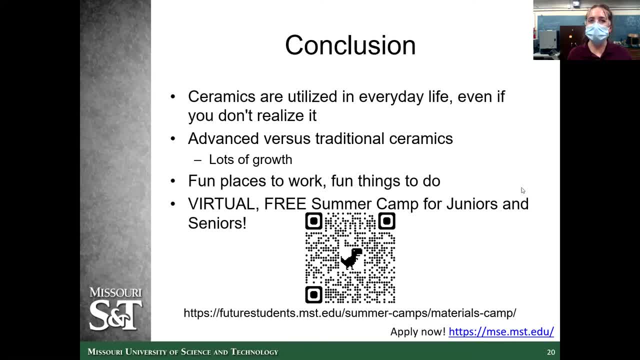 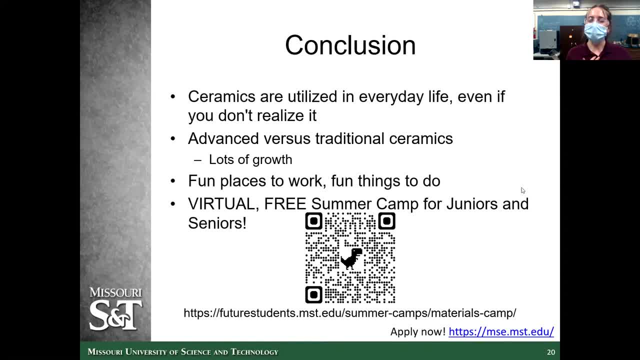 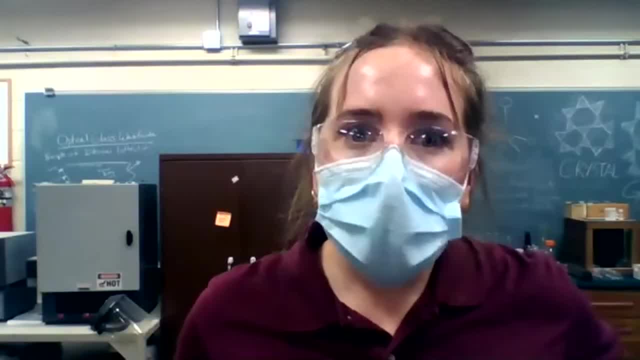 It was. it just did not click for me. I didn't like the material. So after that I was like, oh well, maybe science isn't what it is what I want. Um, and then I took my chemistry class and then all of a sudden it was like, oh, that's what I like, That's what I'm here for, That's. 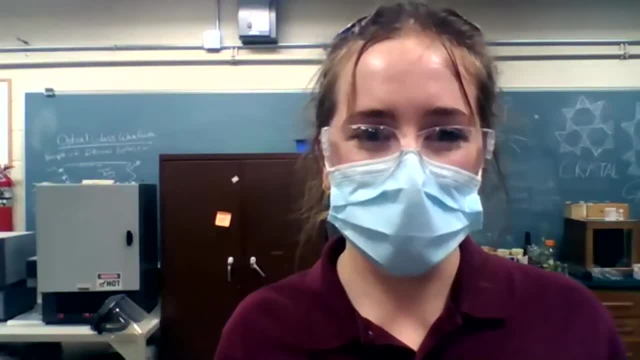 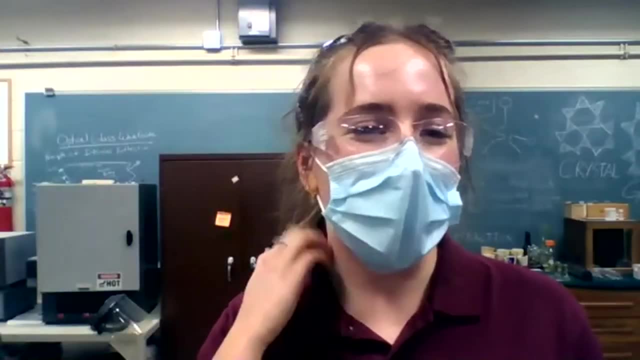 what I really enjoy doing. Um, I really like hands-on aspect. I like being in a lab um, playing with my torches and my chemicals and stuff. I really enjoy all that stuff. Um. so yeah, my favorite science in high school was definitely chemistry. 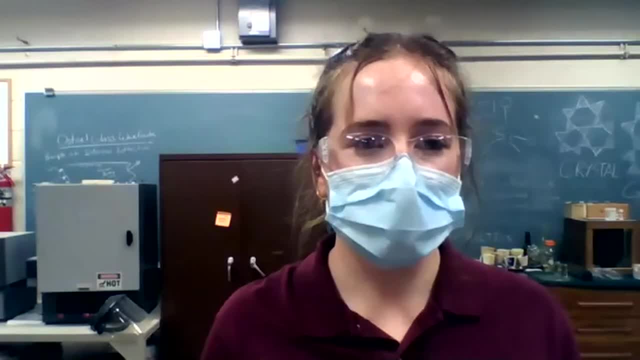 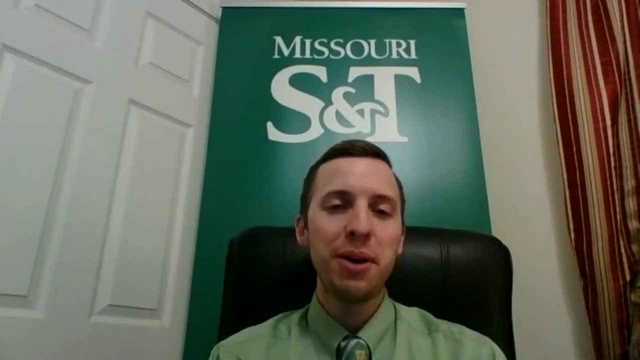 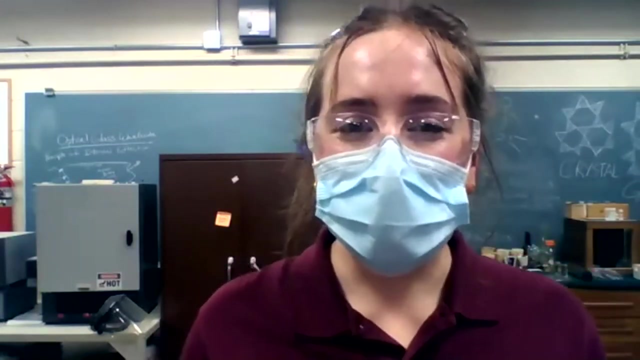 So, as a follow-up question, what is your favorite part about being in the ceramic engineering department at Missouri S&T? Yeah, absolutely So obviously, I'm really passionate about what we do and what we learn, and I really enjoy what we're learning. 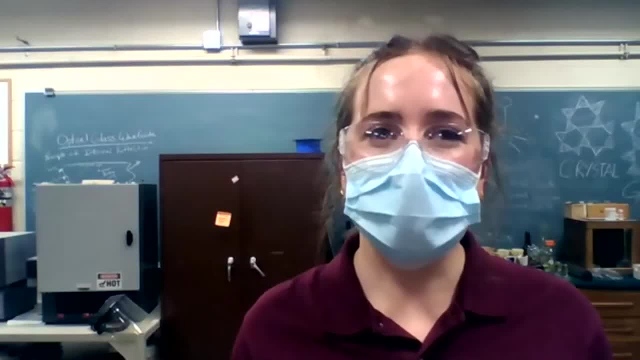 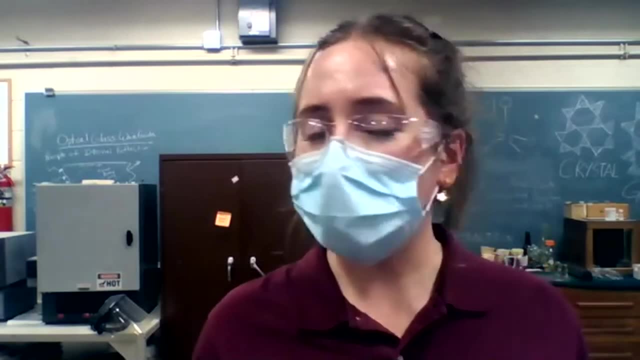 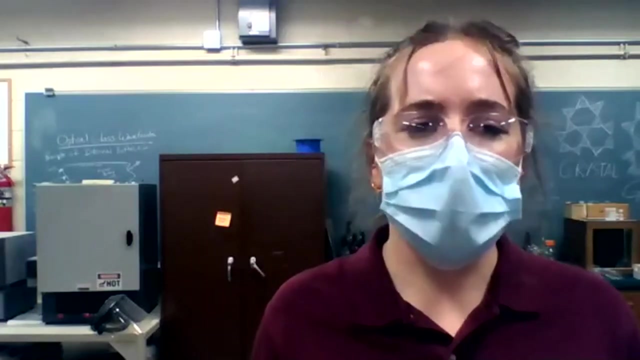 But my favorite part of the ceramic engineering department has to be the relationships I've made through this department. The teachers are amazing. I love all of my professors. They're very understanding, They're fun to be with. I like hanging out with them And on top of that, I really enjoy all my classmates. 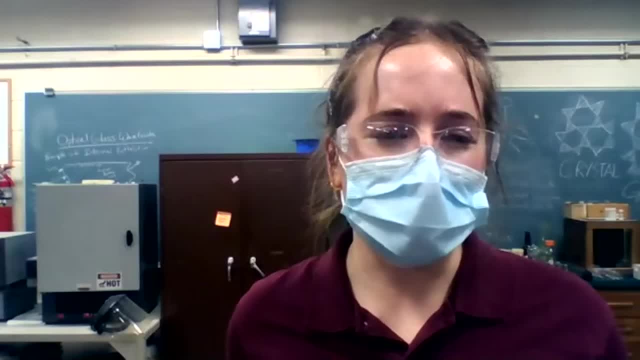 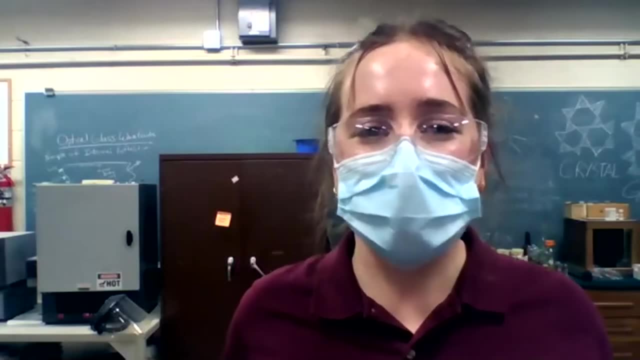 Everyone's very kind. Engineers get a bad rap that they're bad at talking and bad at social skills, But ceramics, ceramic engineers- here they're easy to get along with. I have lots of friends. I've got a lot of really close friends that I've made through this department. 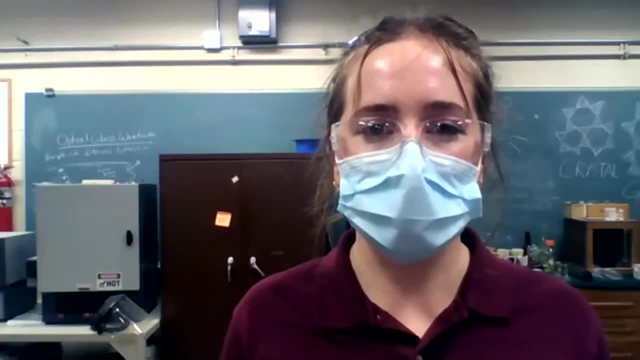 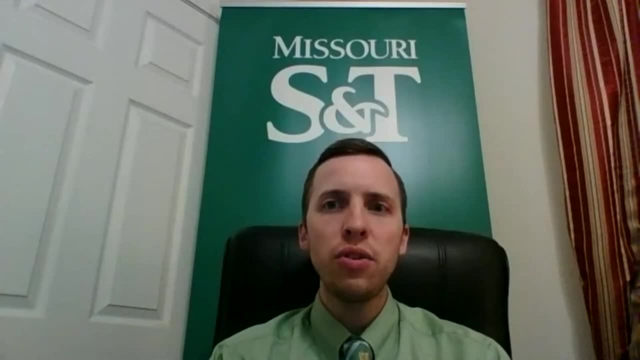 So definitely the relationships are my favorite part of this department. Do you have any advice, Clare, for students who might still be in high school, Things that they can do to help prepare themselves for engineering, for starting off in college? Yeah, absolutely, So we do have that summer camp. 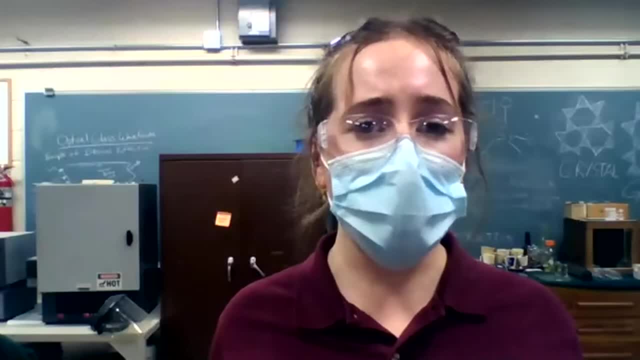 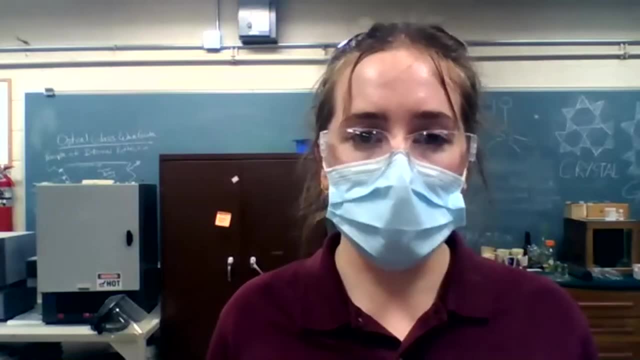 But I know universities across the nation have summer camps that you can go into to get a little bit more hands-on experience, get some of that knowledge that requires you to use your skills. Yeah, absolutely So, we do have that summer camp, But I know universities across the nation have summer camps that you can go into to get a little bit more hands-on experience. 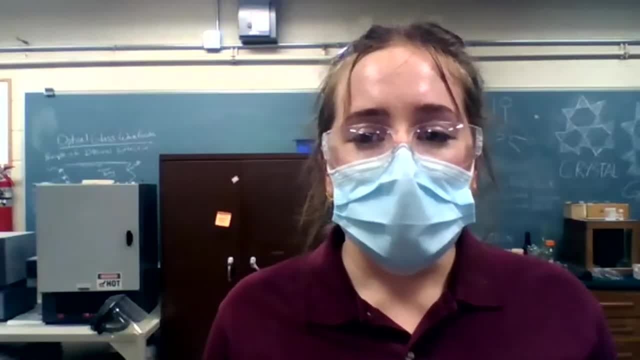 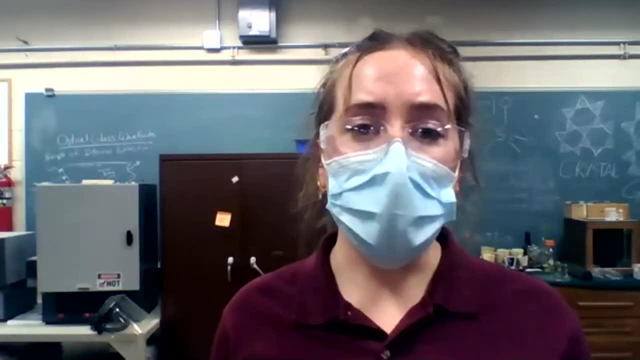 get some of that knowledge that requires you to use your skills. So if you guys are looking at anything engineering related, I would highly, highly, highly recommend getting into it now. I did not have any engineering classes in high school. I didn't have any ceramics classes in high school. 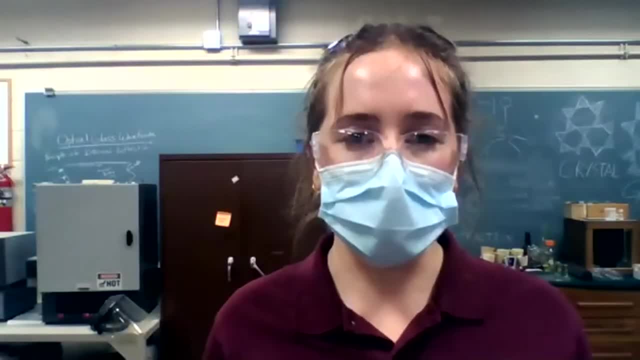 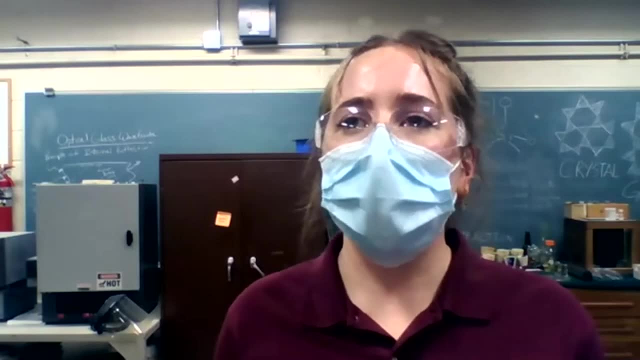 But if I had, I think it would have set me up in a position where I would have not come in as a chemical engineer. I would have known what I wanted to do sooner. So yeah, just get involved right now if you've got engineering clubs, robotics, summer camps. 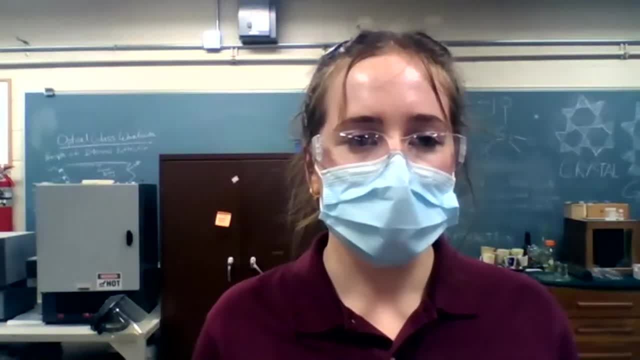 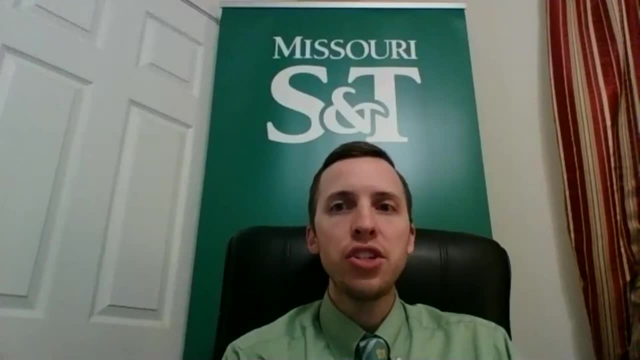 anything you can do, get your hands on it and do it. We have a question as well about the courses that you've taken to get a ceramic engineering degree. If you could kind of talk about what those have looked like, since you are a senior. 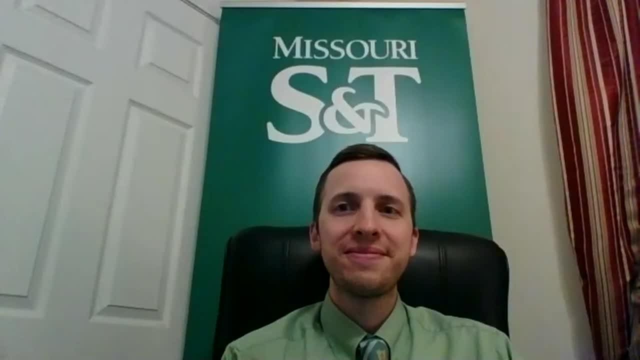 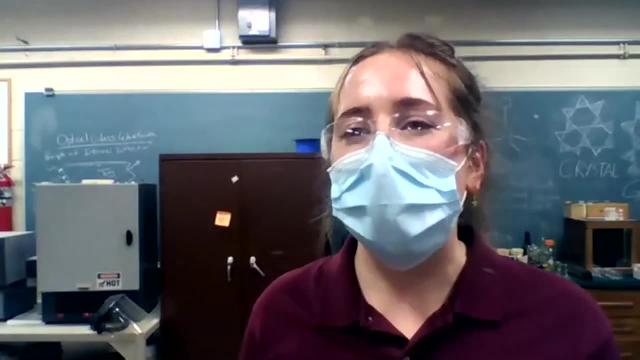 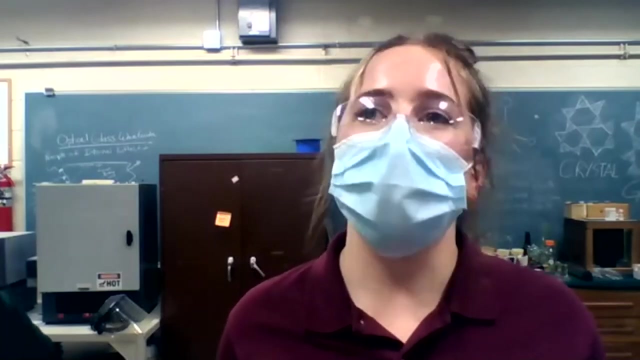 Yeah, yeah for sure. So engineering general education classes don't look like most general education classes at other colleges. We have to take chemistry classes, lots of chemistry classes. I took calculus one, calculus two, calculus three and differential equations. 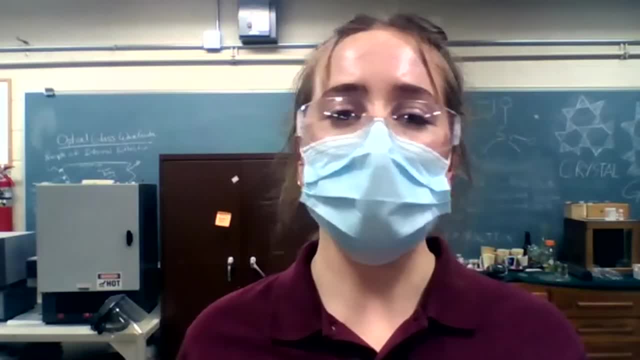 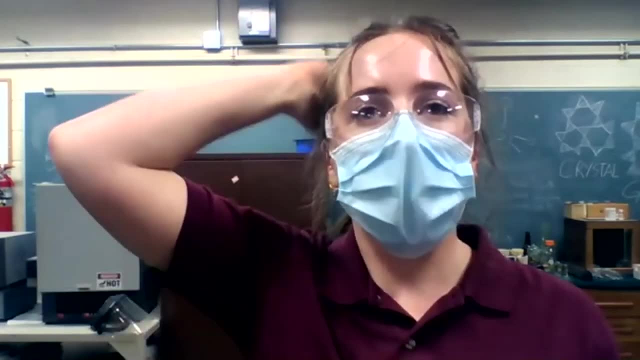 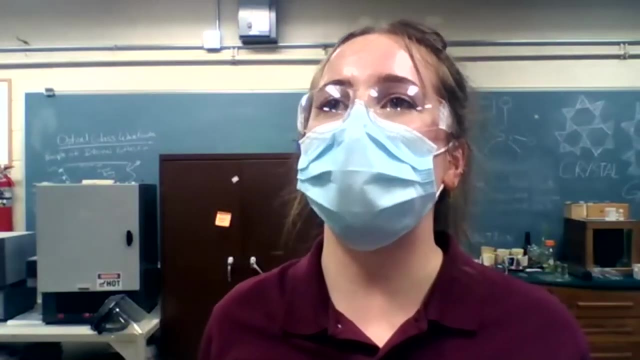 So I took four different math classes to even mark that engineering or mark that box in my engineering degree. That wasn't even ceramics related. I had to take physics one, physics two. For ceramics we have to take modern physics Took. I took like statics, which is like the physics of things. 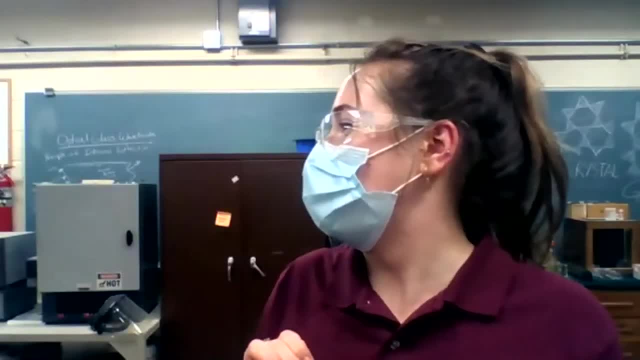 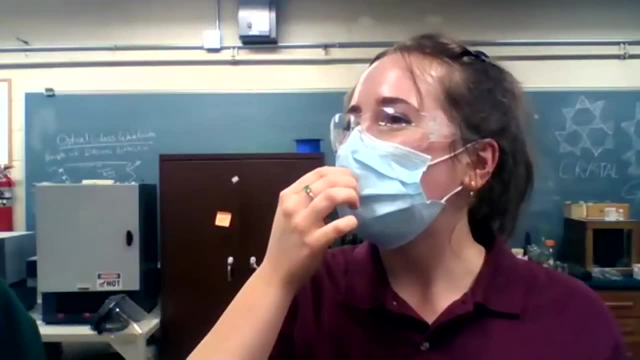 that aren't moving, and then mechanics of materials, which is the physics of things that are moving, kind of. That was a hard class. I don't really remember. I try to block it out. So lots of sciences, lots of math classes. 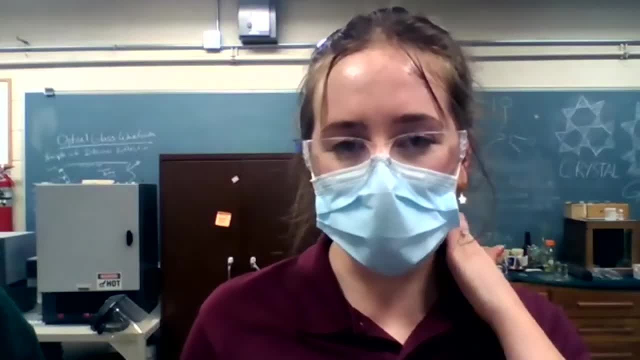 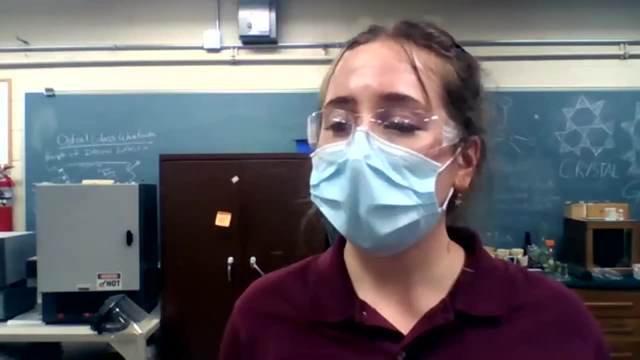 I took all my history and English credits in high school. I got dual credit for those, so I haven't really done any of those in a long time. But ceramics- overly complicated courses. Specifically we have crystallography and that's where you learn about stuff. 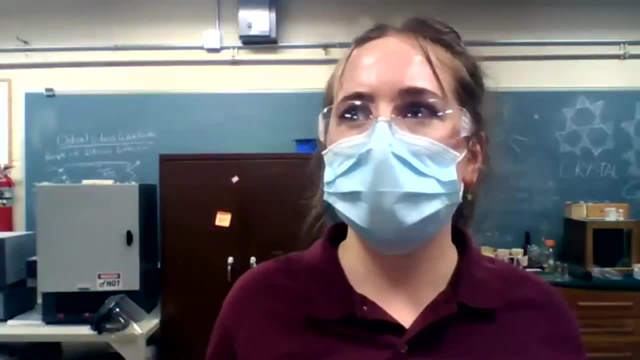 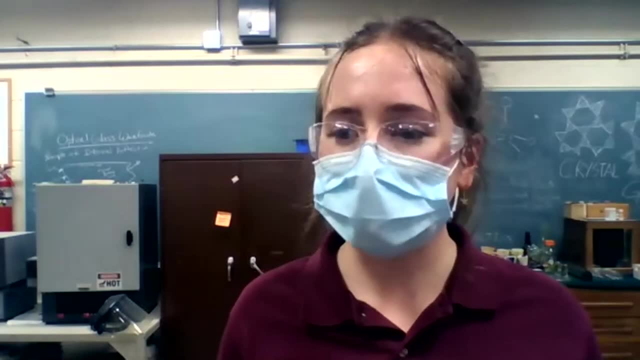 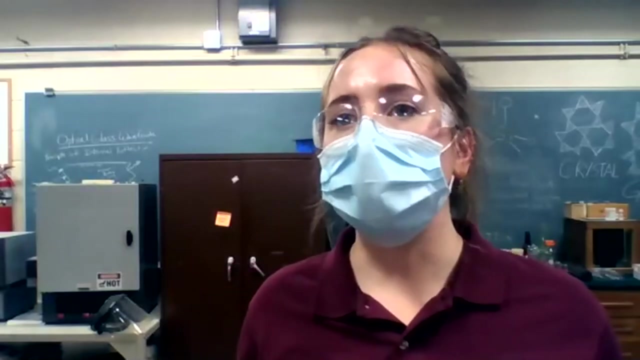 like this, structures and things. We have a lot of different labs. So your sophomore year and your junior year, you're required to take a lab every semester And that's when you're actually in the lab performing experiments, writing lab reports, doing. 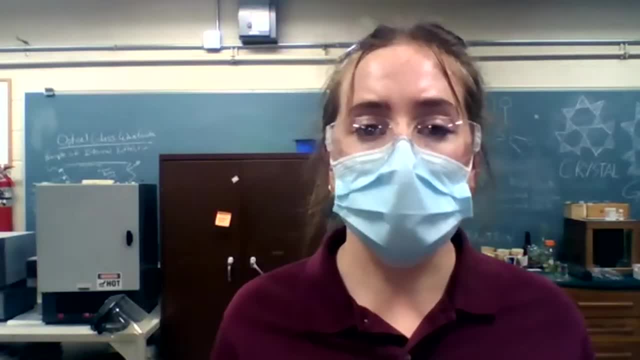 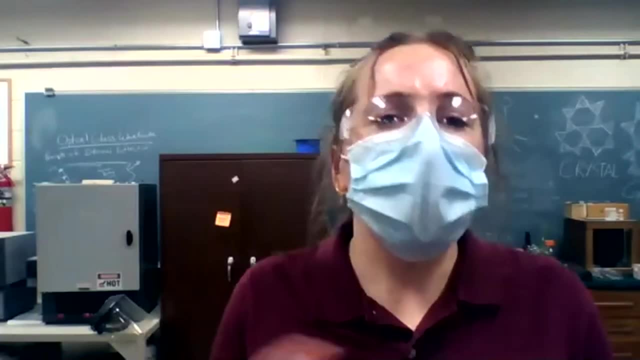 presentations. So those were, Those were because they were so hands-on- like I said, I really enjoy that hands-on aspect- and then a lot of like the nitty-gritty, like the electrical properties of ceramics, kind of like I was talking. 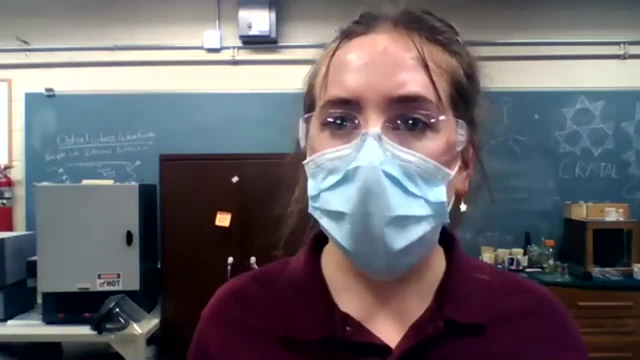 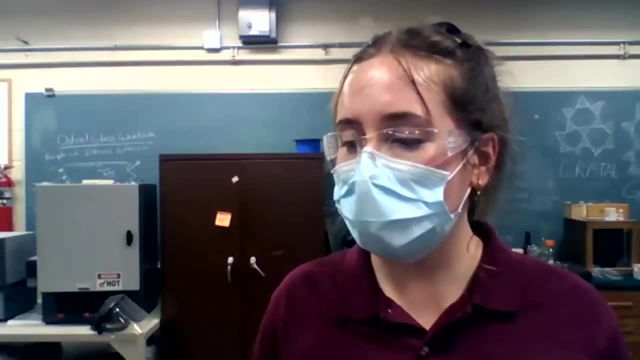 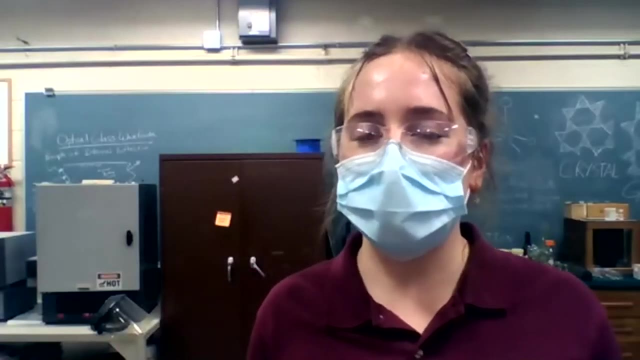 about with the piezoelectrics, the mechanical properties, so how we can control that microstructure to make really, really strong, high-strength structural ceramics. so a lot of really specialized classes, but yeah, there's like there's a whole bunch, there's a lot of. 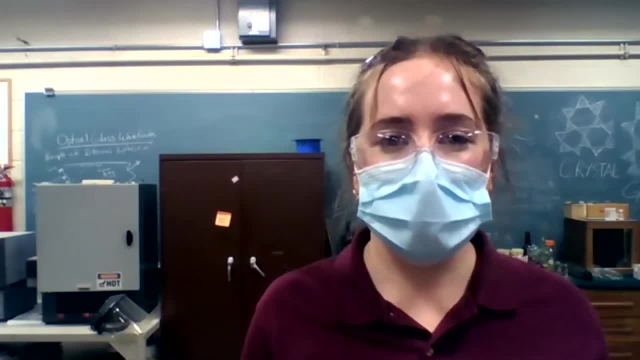 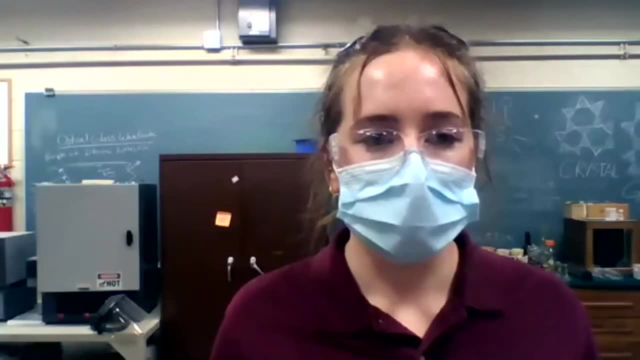 different technical electives you can take. if you're interested in one type of ceramics over another, There's a lot of technical electives you can take to dig deeper into those kind of courses. Something else that I'll point out that Claire had touched on, is those general sort of courses. 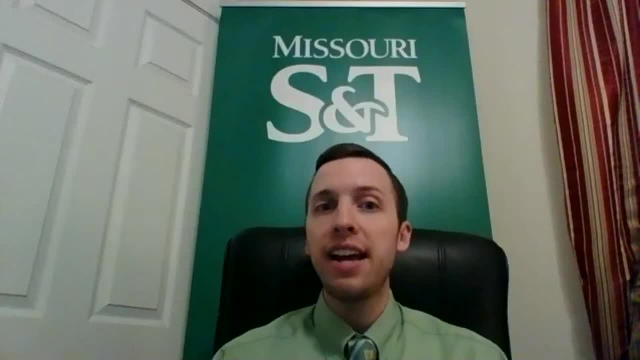 that all of our engineers take. so at S&T we have 15 kinds of engineering and the first year for them is the same across the board. It's taking Calculus 1, it's taking Chemistry 1, taking Physics 1, so it does give you that. 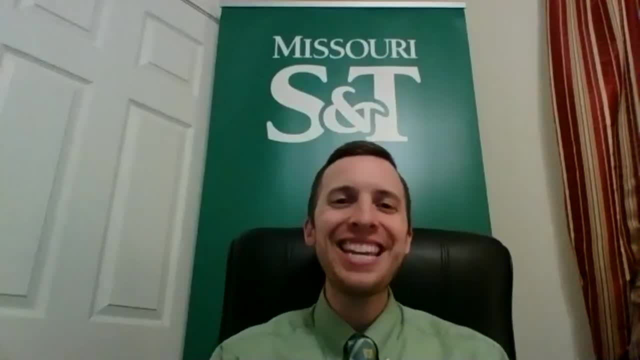 flexibility if you like, Claire, come in thinking you want a certain type of engineering and then change your mind that you're really not going to fall too far behind because of that first year being a common year. Yeah, yeah, so when I did change my major, I changed my major before I. 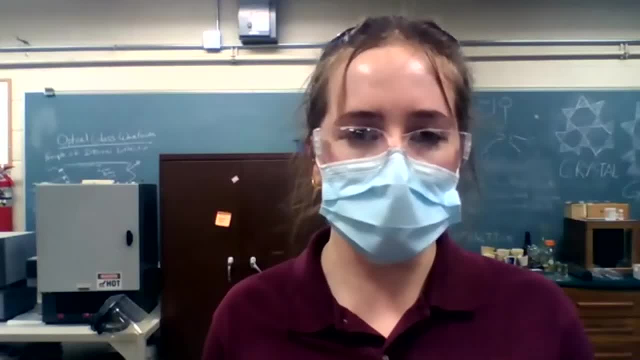 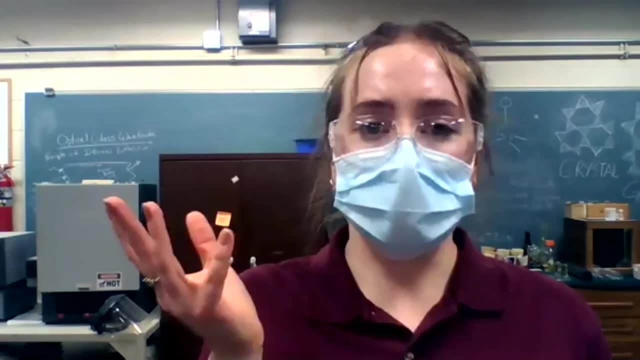 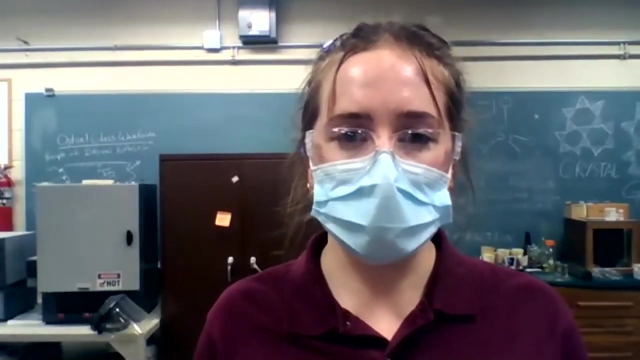 started my sophomore year, but it didn't set me back at all because I hadn't actually gotten into any of those chemical engineering courses and, like Tyler was saying, as a freshman you come in, you start off with a freshman engineering class and that's where you learn about all the different types of 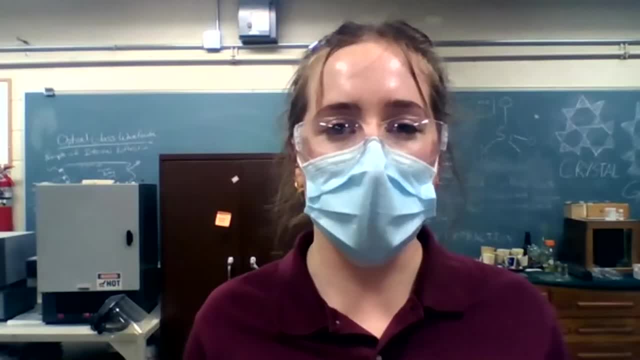 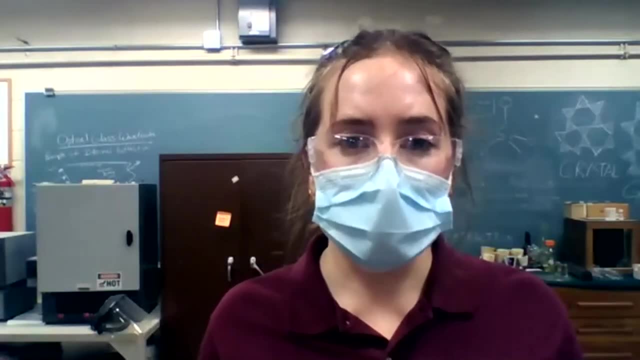 engineering. They go every week. you go into a different type of engineering and you write a little report on it. you learn more about it. so S&T really sets you up really well to choose the kind of engineering that you're most interested in. 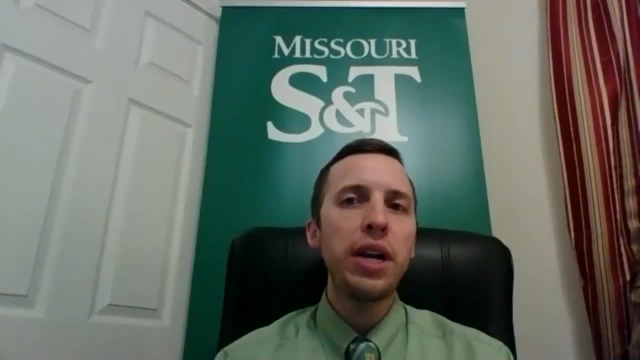 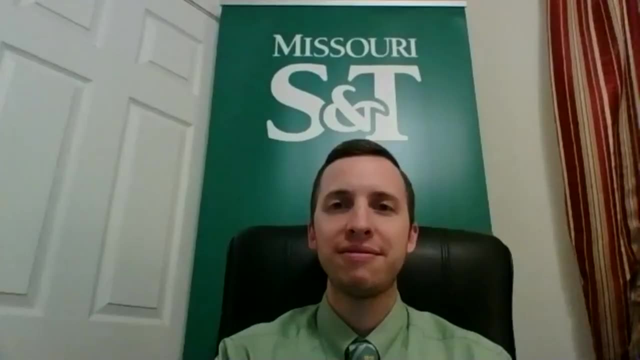 The next question for you, Claire, is: could you talk about what you're wanting to do after graduation? Yeah, absolutely So. I graduate next semester, but I'm actually staying at S&T. I'm going to be here for a couple more years. I'm going to do my 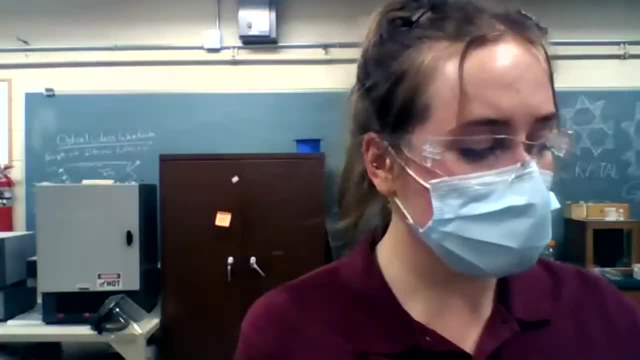 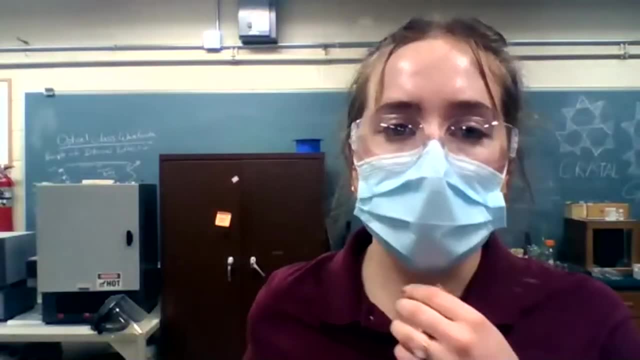 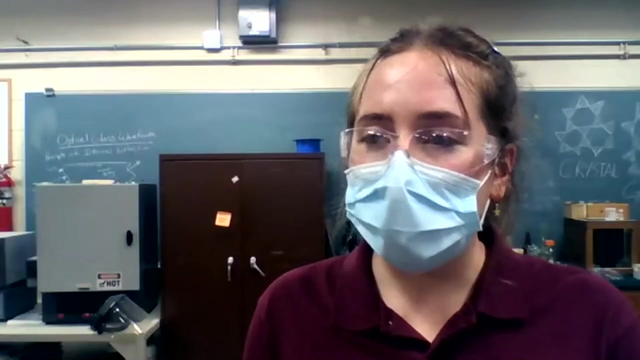 master's. Currently I'm looking into getting into more of the glass side of ceramics or the structural side. so I haven't done a whole lot of digging into it yet, since I still got a little bit before I do graduate. but I'll be here for a while and then after that I'm going to head. 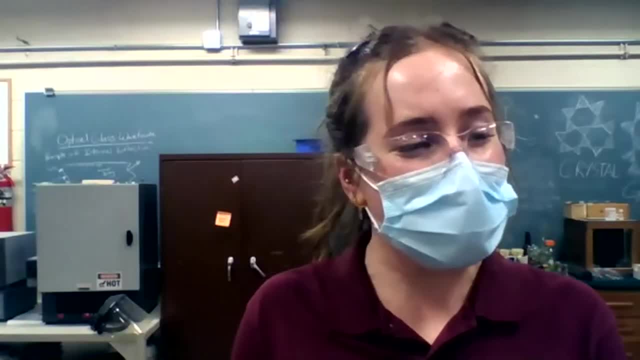 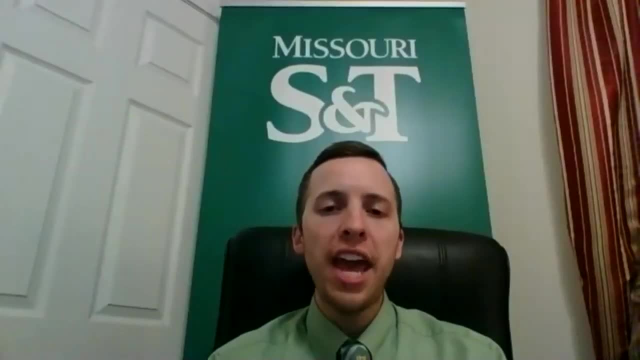 back to Kansas City and work a little bit, pay off some debt and then hopefully find my dream job. You mentioned that you had an internship or a co-op, and then I also recall you saying how you were working with Brewer Science. Would you mind talking about your experience through that co-op? 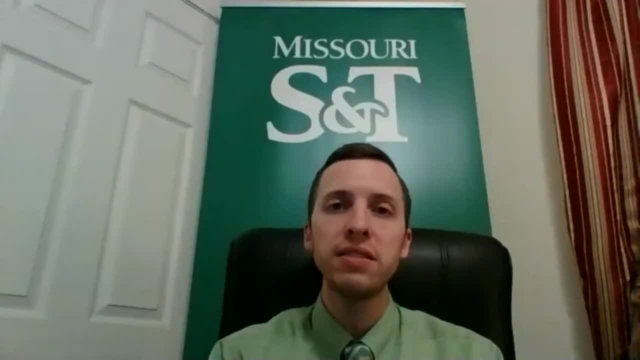 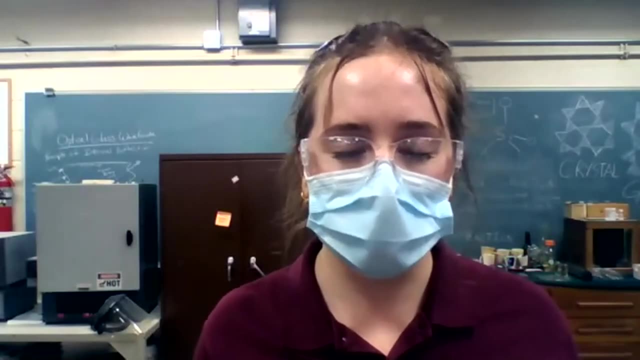 or internship or with Brewer Science. Yeah, absolutely So. I worked with GE Aviation. I took a semester off last semester. I went and worked full-time with GE Aviation. I was in Madisonville, Kentucky and it's kind of hard for me to describe exactly, but I was in Madisonville Kentucky. 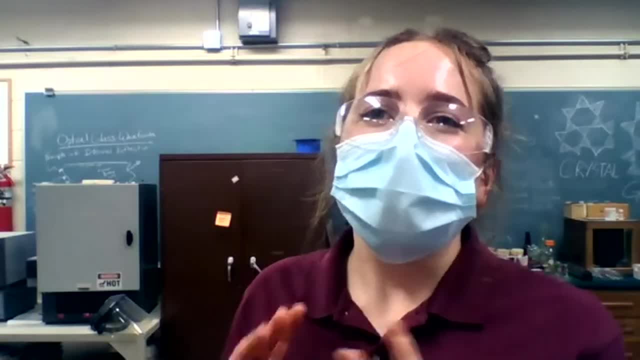 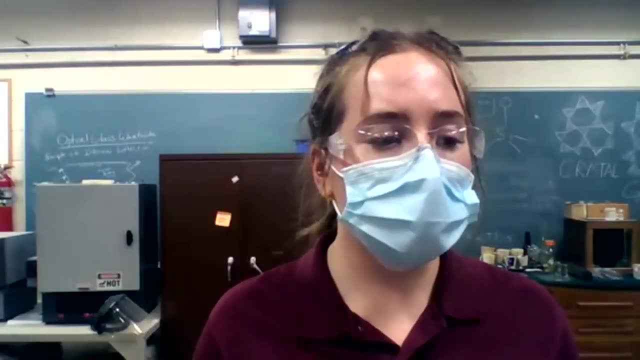 and so I was able to go do my job description, because everything got thrown off because of Covid. Thankfully I was still able to go and work in person, so I was there the whole three months working with them in person. so I'm very grateful for that. very lucky with that one. 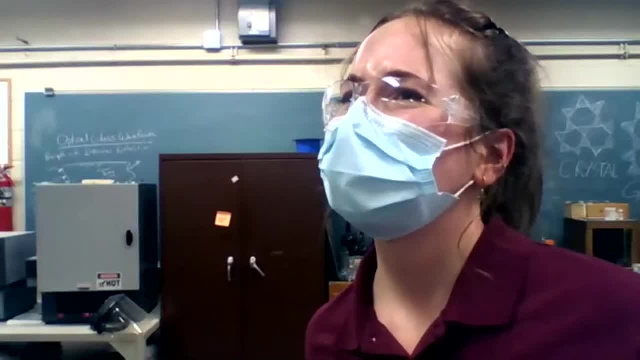 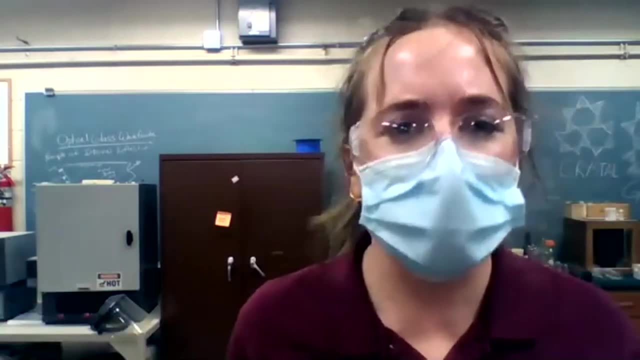 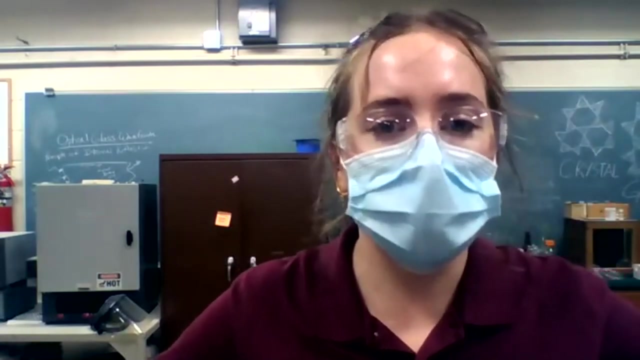 but I did a lot of linework manufacturing engineering, So I did a lot of that stuff last semester. Right now I am working with Brewer Science And, like I said, they're a semiconductor company and I'm doing quality engineering through them. 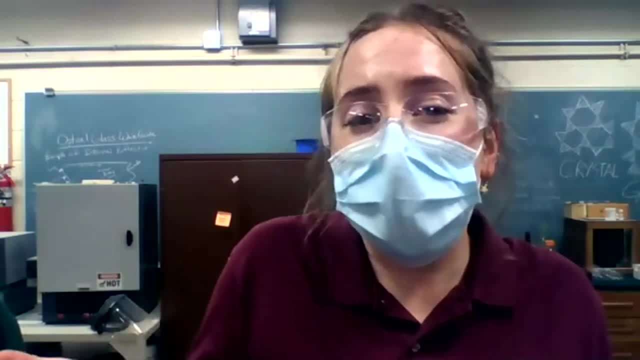 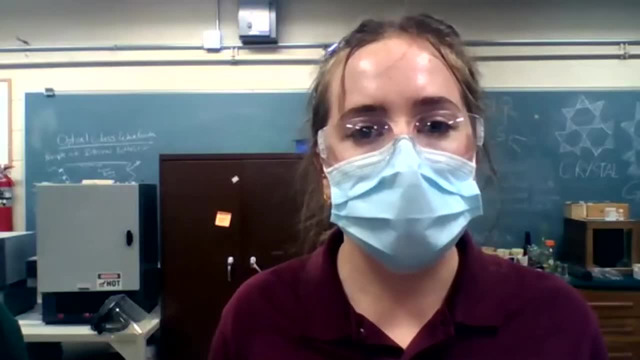 So, obviously, manufacturing, the quality engineering service can go anywhere. You can do anything you want with it. And then this summer I'm working with Catalan, which is a pharmaceutical company, And I'll be doing process engineering with them. So, yeah, I really like it. 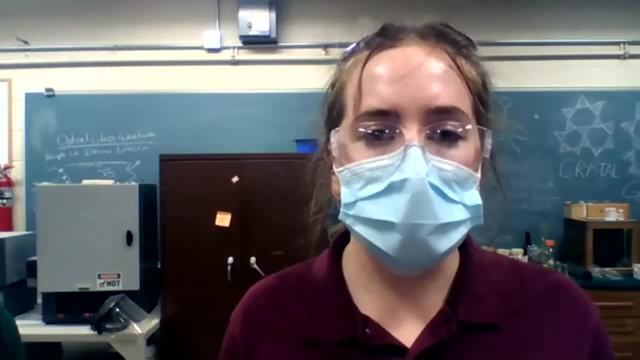 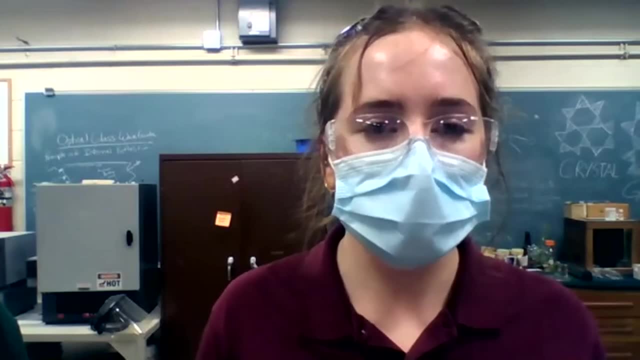 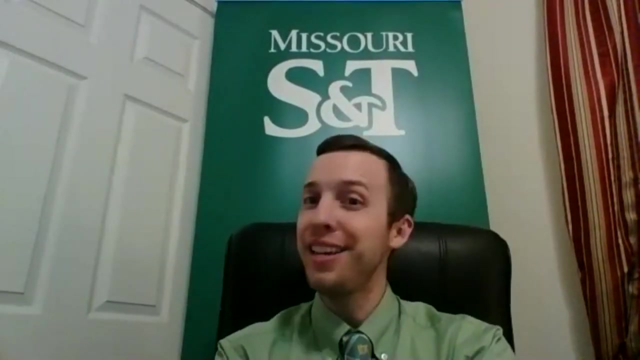 It's Brewer right now is all online, So I'm just working from home and working on my computer. But that's been good. That's been a lot more hands on kind of stuff than GE was. We have a question in the chat for you, Claire, about what is your dream job. 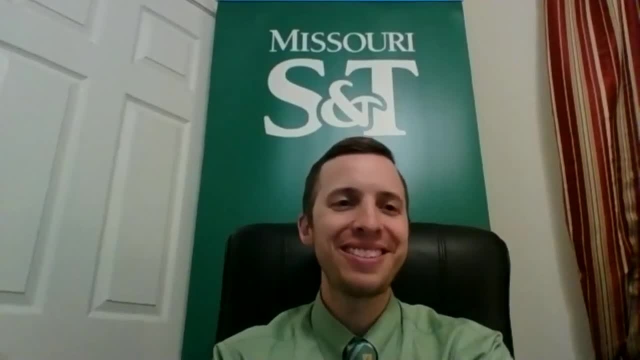 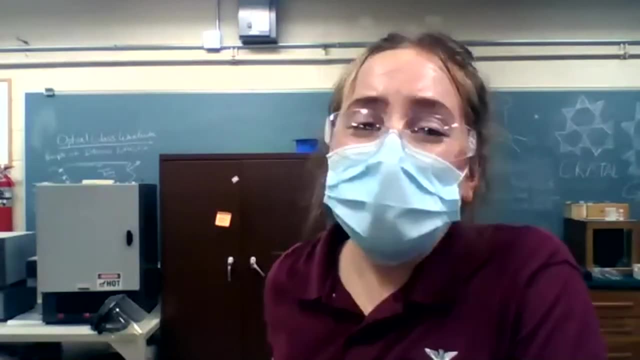 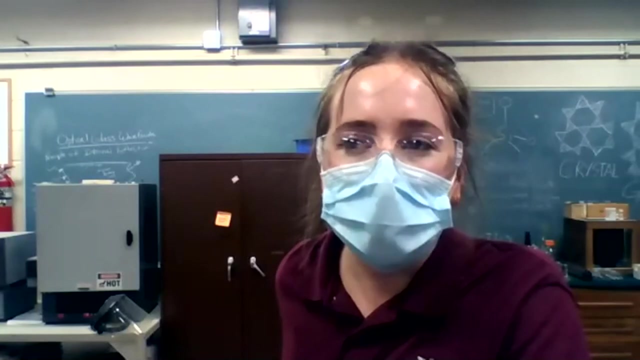 So after you would graduate with that master's? Oh, that's a really really good question. I do enjoy being in the lab and doing those hands on experiments, So I think somewhere in the research and development area would be really, really cool. I like to do the inventing, the research. 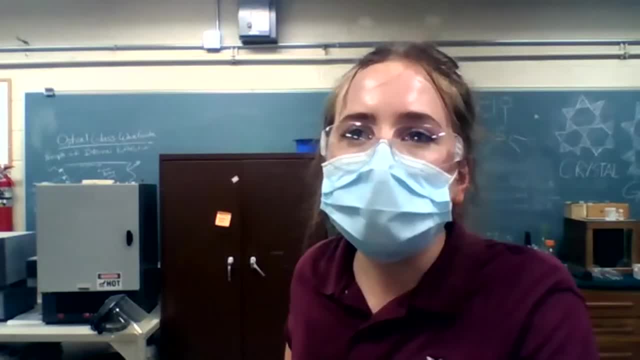 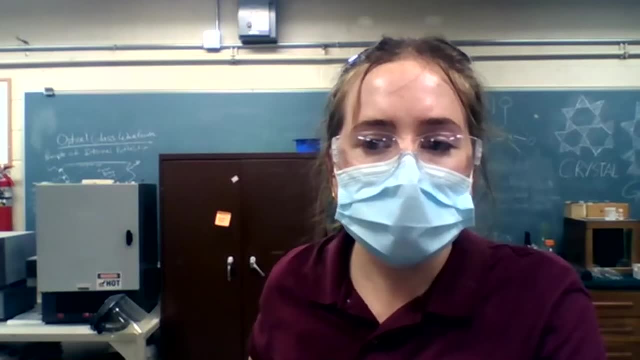 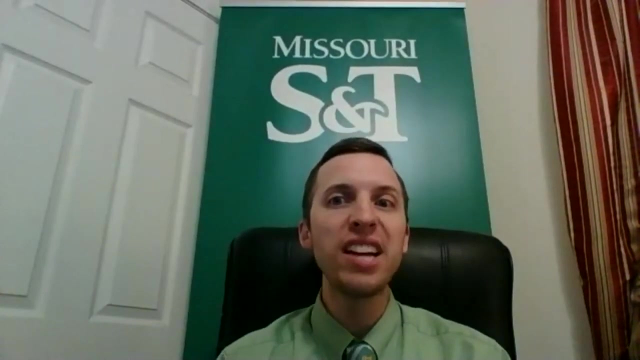 the let's come up with new stuff, Let's solve this problem. So, somewhere in the research and development field, I think would be very, very cool, All right, So someone was wanting to know if you could explain what process engineers do. 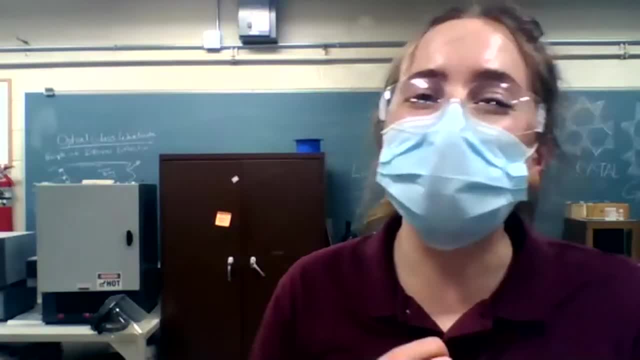 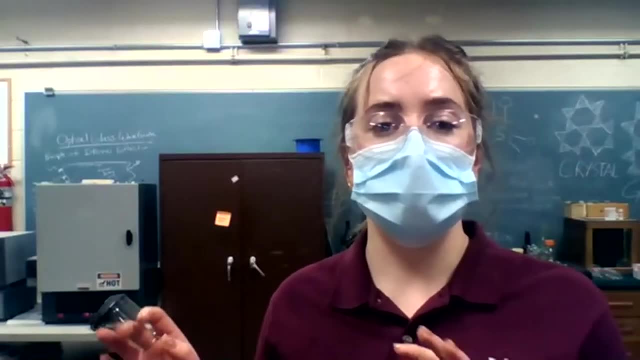 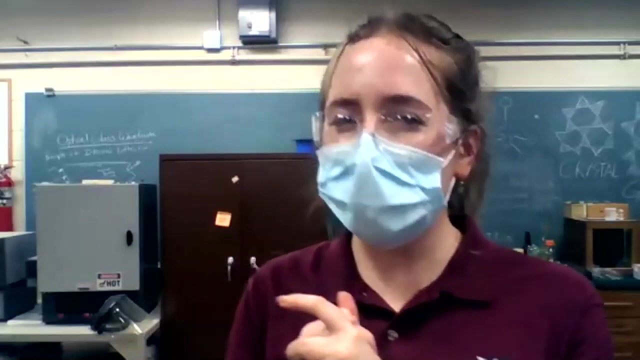 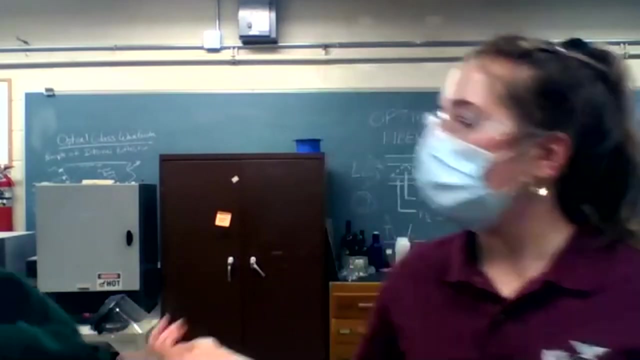 Yeah, yeah. So I haven't started that position just yet. can't give you specifics, um, but from what i understand, they oversee the process of products going from raw material all the way through final product. so i'm pretty sure what i'll be doing with this summer is, um, oh yeah, do you want to talk about it? yeah, go ahead, yeah, okay. 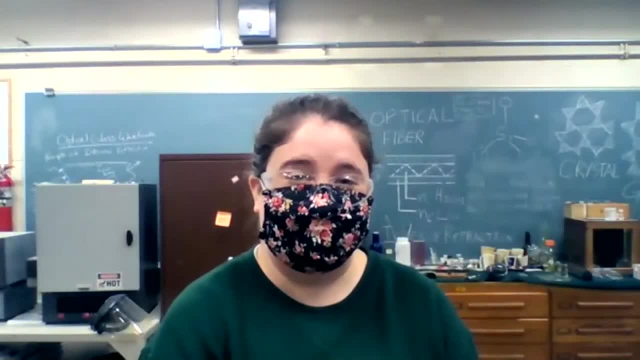 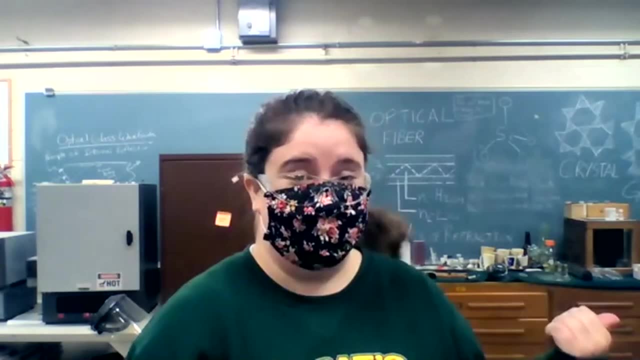 so actually i did process engineering on my co-op, so i was at san diego and we were doing manufacturing, um, and so what process engineering is you're looking at? um, like um? claire was saying how you have like a raw powder to a solid, like ceramic piece, and so there's a lot of steps in. 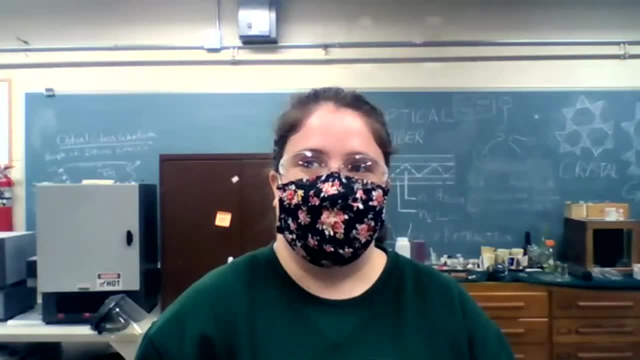 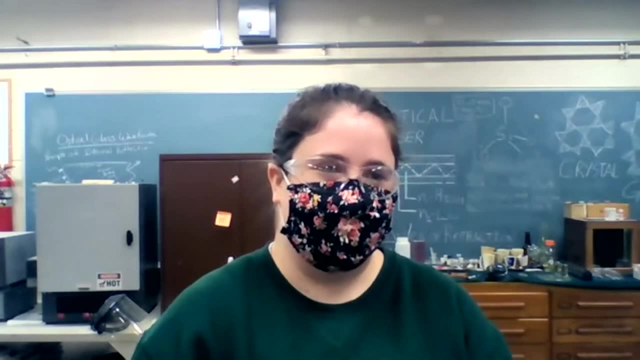 between that happen with that. so you have to. your material has to have like a certain phase and you have to put it in the furnace a couple times. you have to change what your particles look like. so because your powder is like tiny little grains but depending on what shape and what like your 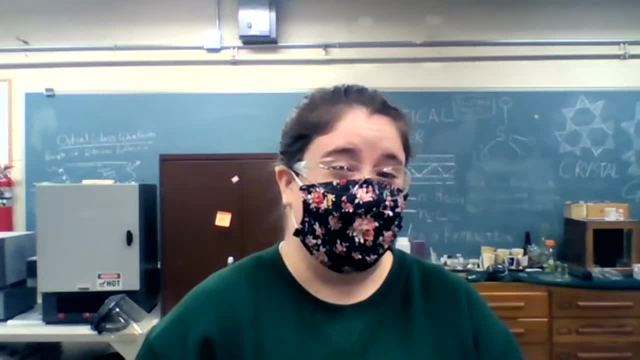 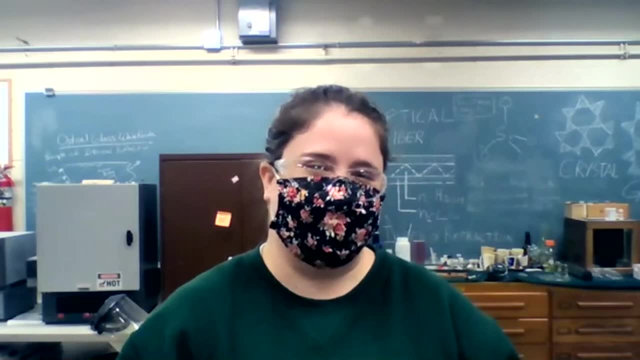 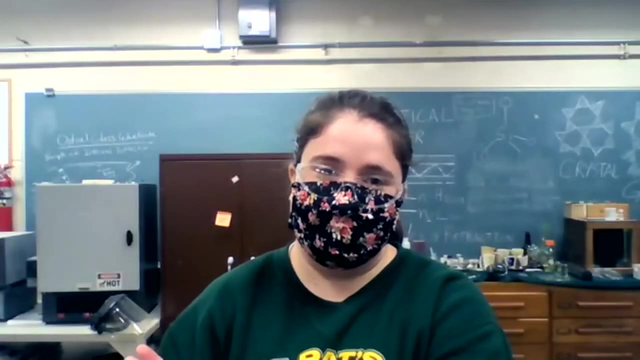 morphology and how, like what size it is, um, it really impacts your material properties when you center it into a full, um solid piece. so you look at each of those steps. there's actually like we have like 16 different steps, from like raw powder to like the final, like centered piece, and so you there's like so many factors for each of those. 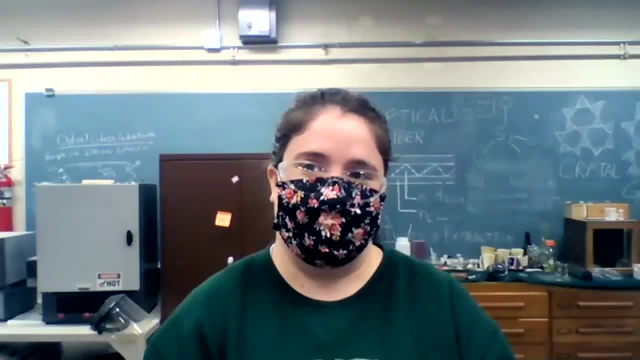 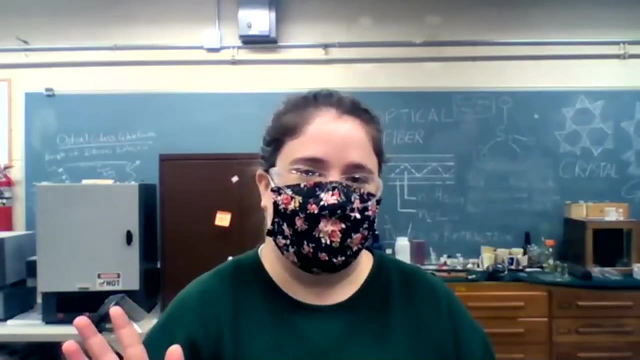 steps and so you're working on each of those factors to make sure that your final product is good, because a lot of times the ceramics you get a lot of cracking. so you have to um troubleshoot where your cracks are coming from, because you have, like you can have, over 30 different factors and all of them could be causing your cracking. 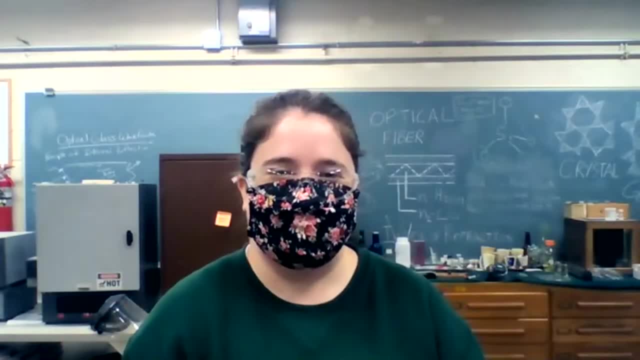 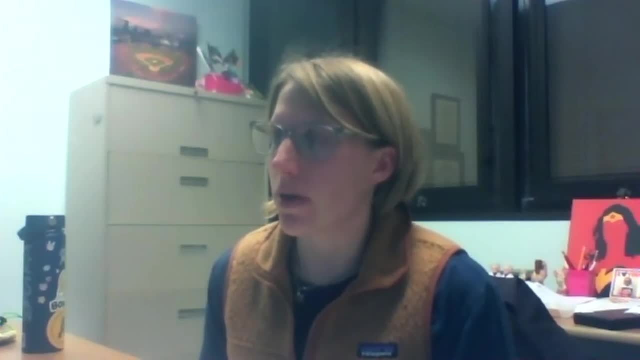 but if only one of them is actually the culprit, so it becomes really complicated. appreciate you guys taking the time tonight to come and learn about ceramic engineering. um, we really hope that you want to come and join us. we'd love to have you in our department, um.